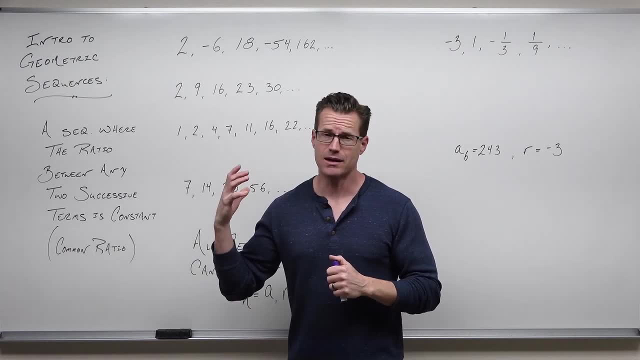 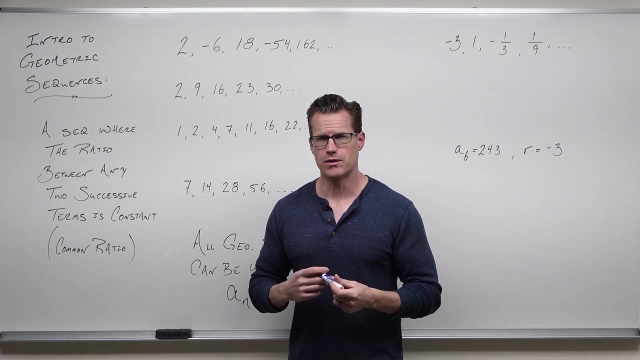 geometric sequence on which it's based. So we'll talk about what exactly a geometric sequence means, how it's built, how to figure them out. from one term, or maybe two terms, deal with what the sequence should look like formulaically, and then in the next video we'll talk about the 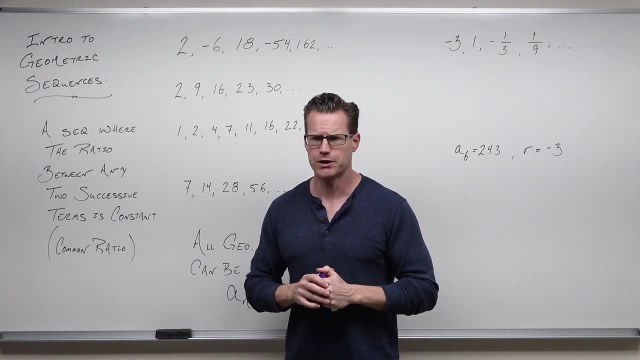 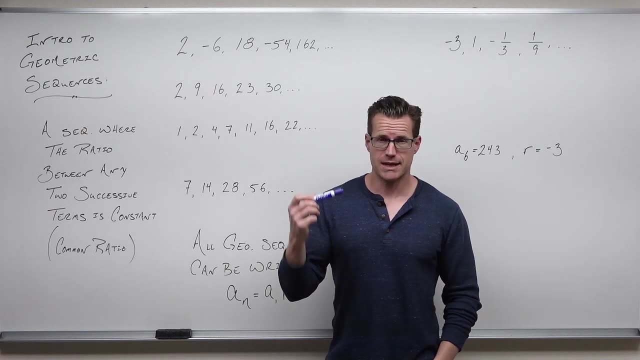 series. how to add those terms up? There's some really interesting formulas that we get. We'll talk about something called convergence and divergence of a series. That's about it. So what a geometric sequence is. it's actually quite similar to an arithmetic sequence. 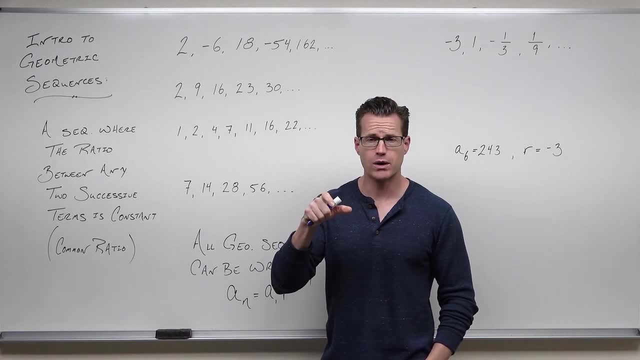 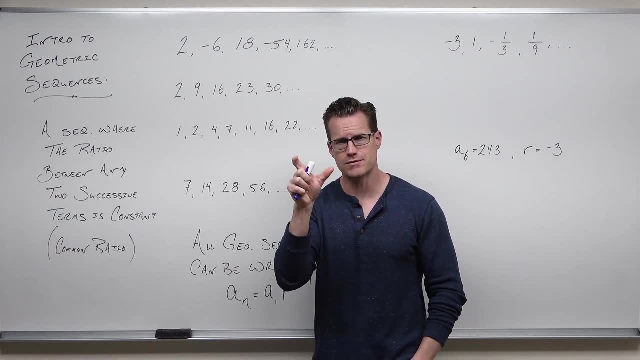 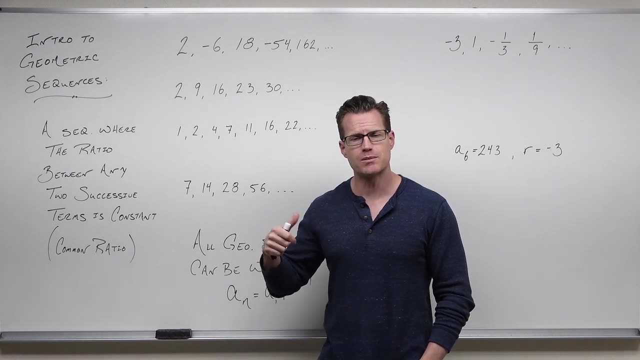 had what was called a common difference, which meant if you took two successive terms and you subtracted them, you can do the same thing over and over and over again. That was what number you're adding. Well, we have something similar, except instead of adding the same number over. 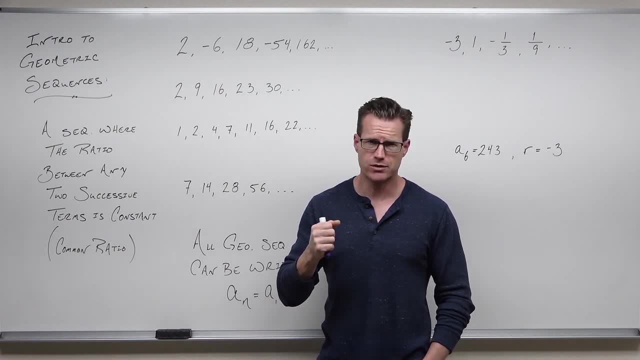 and over and over again. we're multiplying. So geometric sequences and series are built on the idea of taking some starting number and multiplying to get to the next term and the next term by the number, over and over and over. Now that number that you're multiplying by is called the common. 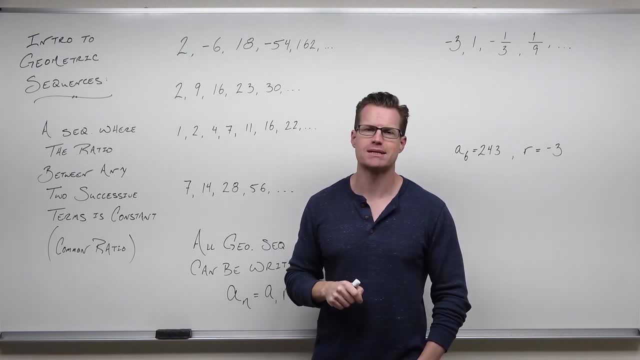 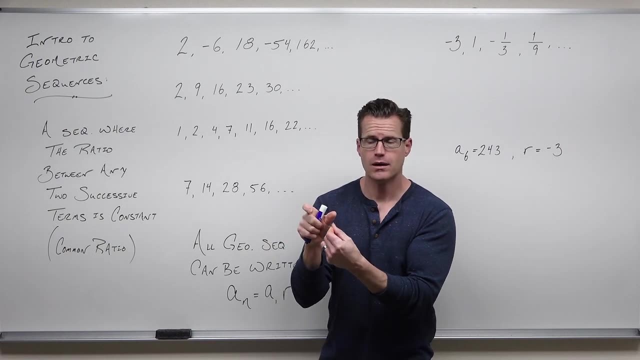 ratio And the idea goes back to an arithmetic sequence and says: all right, arithmetic sequence, if I took two terms and I subtracted, that's going to be the number that I'm actually adding. Well, if I take two terms here and I divide them- the second term by the first term or the third- 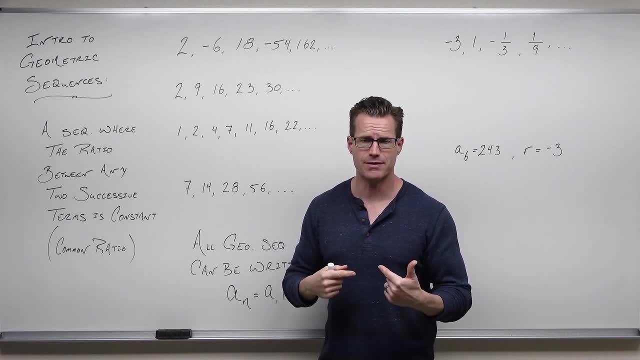 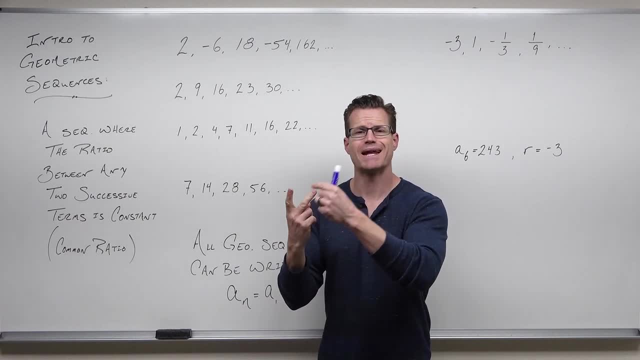 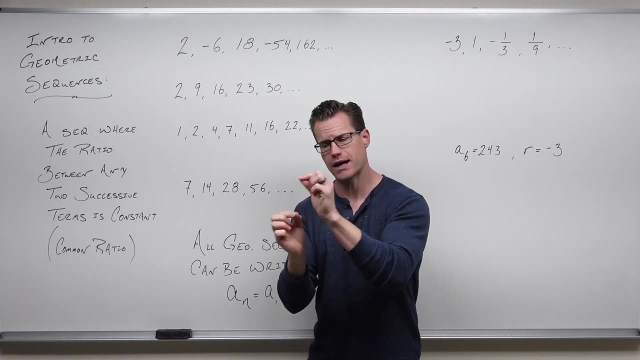 You need to know what number you are multiplying to get to the next term and every subsequent term after that. That number that you're multiplying is called the common ratio, because when you divide two successive terms, it's going to give you the same fraction every time. Now, sometimes we get a. 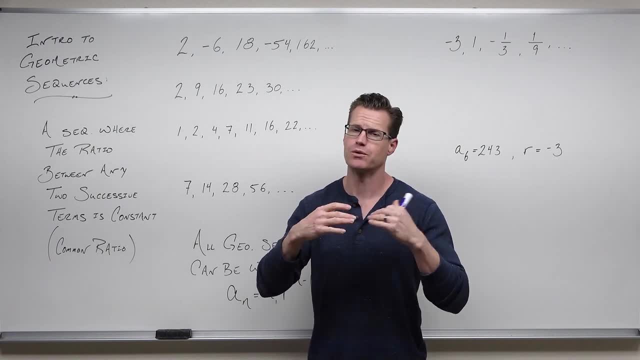 whole number, but it still is a fraction. Common, same ratio fraction. I hope you're seeing the similarity between this and arithmetic sequences. They're built the same way. Instead of adding over and over, we are multiplying over and over and over again. 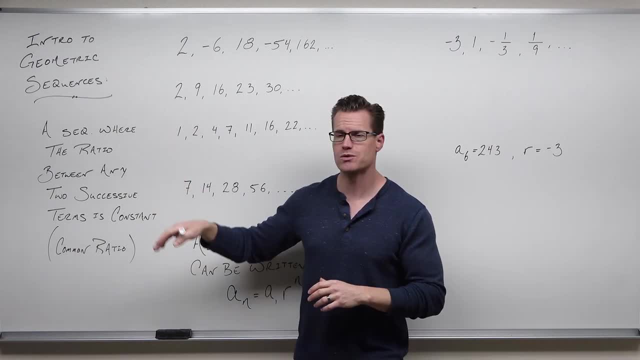 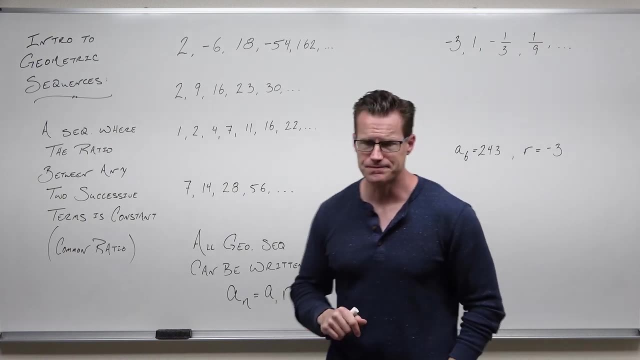 You still need to know the starting spot, And that's what all this says. So it's a sequence, or the ratio between any two successive terms is constant, called the common ratio. So what we're going to do, we're going to take a look at these examples, We're going to figure out which ones. 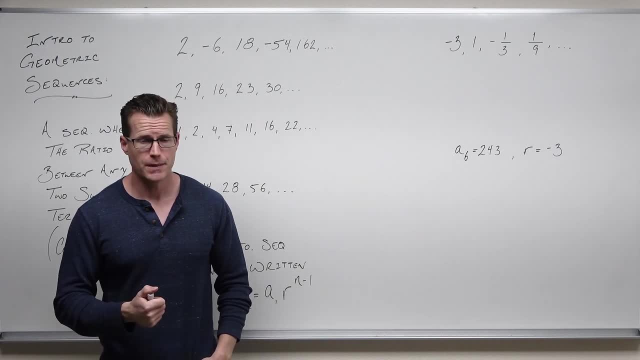 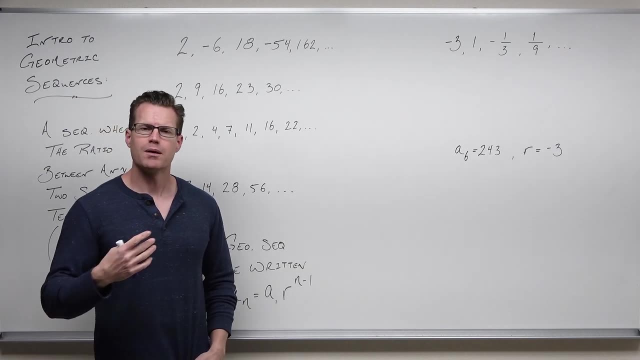 are arithmetic, which ones are geometric and which ones are neither. Sometimes you have a sequence that has a definite pattern, but you don't exactly know. Well, you maybe do know what it is, but you don't have the ability to call it. 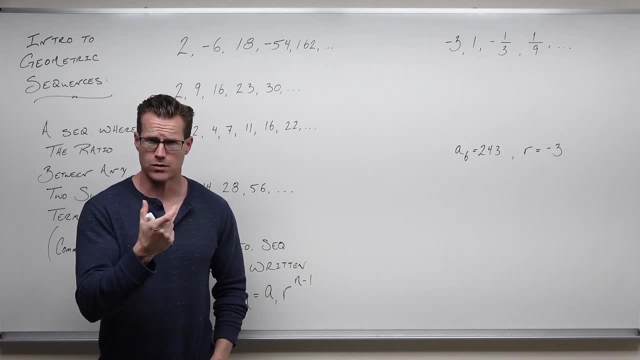 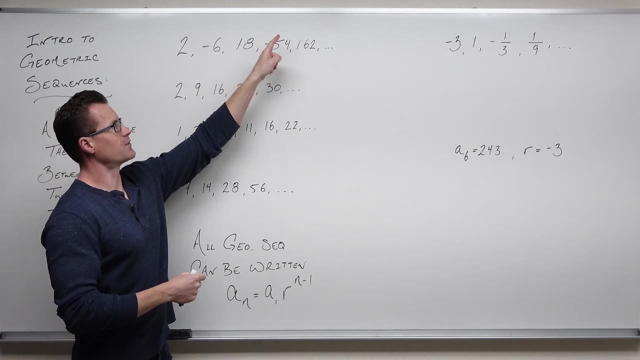 Arithmetic or geometric, because it doesn't fit that that model, And so let's take a look at these. When we take a look at something like this: 2, negative 6, 18, negative 54, 162.. If we're 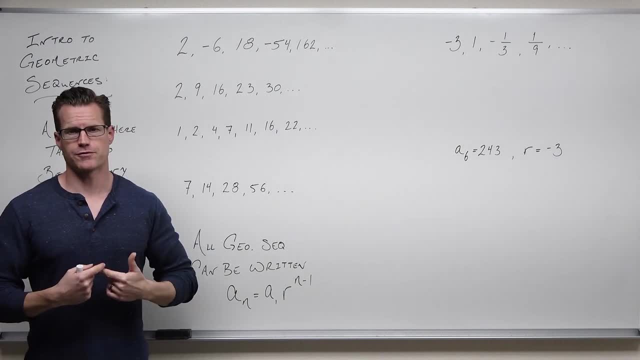 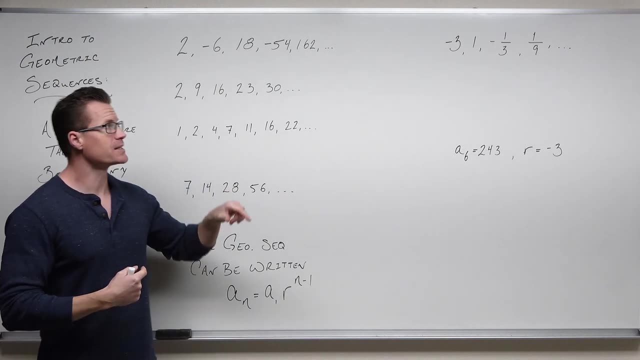 trying to classify this. maybe we try to figure out if it's arithmetic first. Arithmetic means that you're adding the same number over and over again. How you can always determine if you have an arithmetic sequence is: take two terms and subtract them. This minus this, So negative 6. 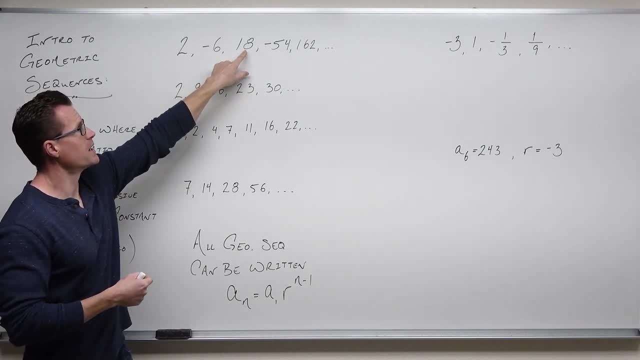 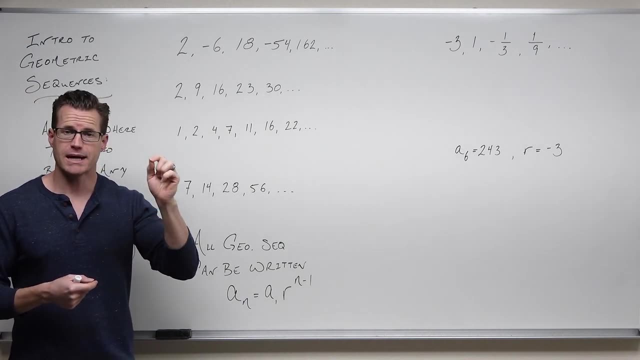 minus 2 is negative 8.. Okay, Take these two terms: 18 minus negative 6 is not negative 8.. That's 24.. Well, if you don't get the same common difference, then you're not adding the same number over and over again. 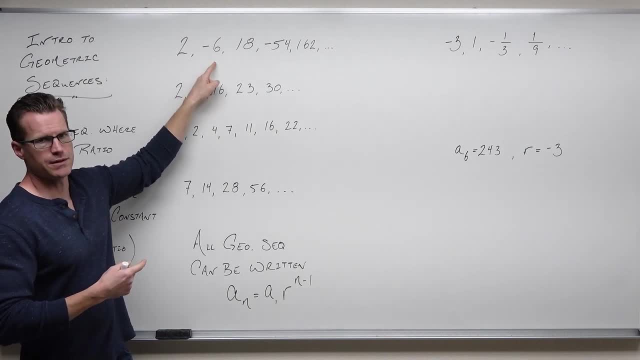 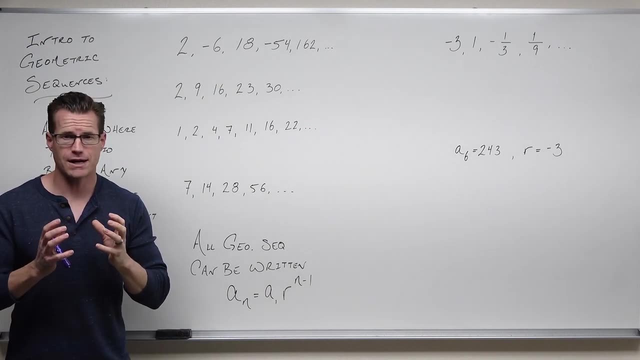 Obviously we're not doing that. If I had to add from 2 to negative 6,, well, that would be negative 8.. And then negative 6 to 18, I'd have to add, I'd have to add 24. Well, that's definitely not. 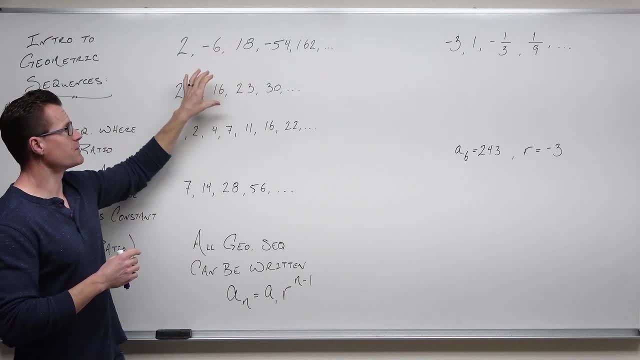 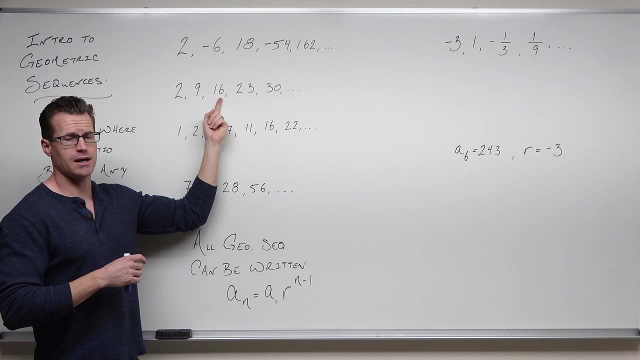 a common difference. This is not arithmetic. Let's see if this one's arithmetic. From 2 to 9, I'm adding. let's see 7.. From 9 to 16, I'm adding 7.. From 16 to 23,: I'm adding 7.. From 23 to: 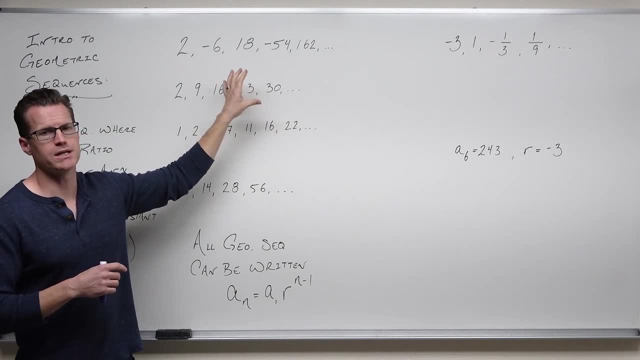 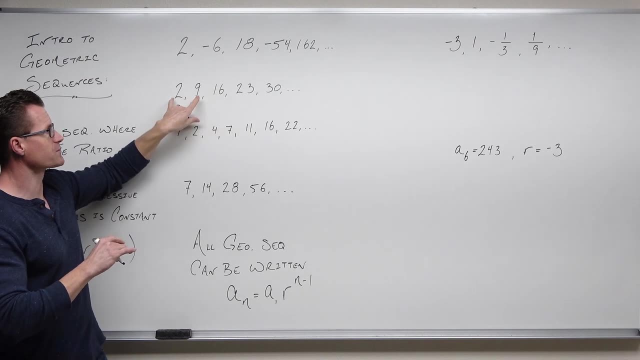 30, I'm adding 7.. This is arithmetic. This would be a sequence like we dealt with two videos ago. This is an arithmetic sequence because of the common difference If I were to subtract two successive terms: 9 minus 2, 7.. 16 minus 9, 7.. 23 minus 16, 7.. 30 minus 23,, 7.. Do you see how? 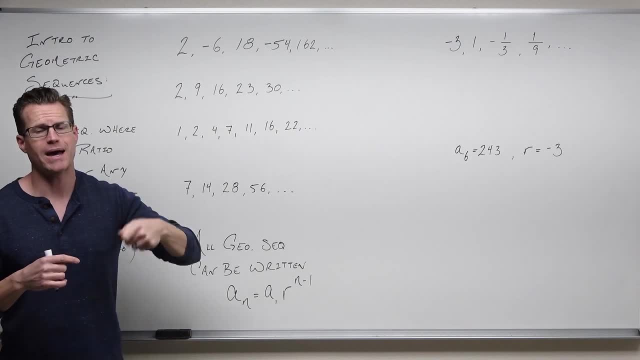 taking two terms and subtracting them is giving me the number. I'm adding, I'm adding 7.. From 9 to 16, I'm adding 7.. Remember, I'm adding over and over and over again. This would be arithmetic. 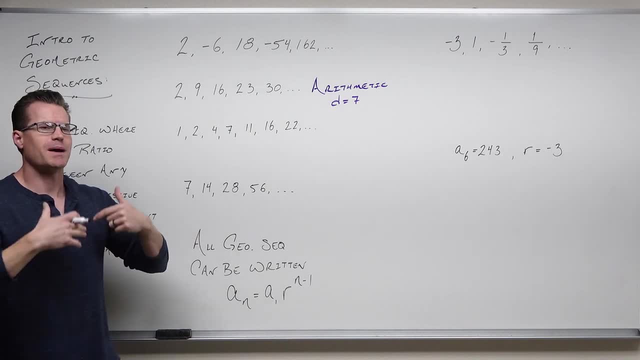 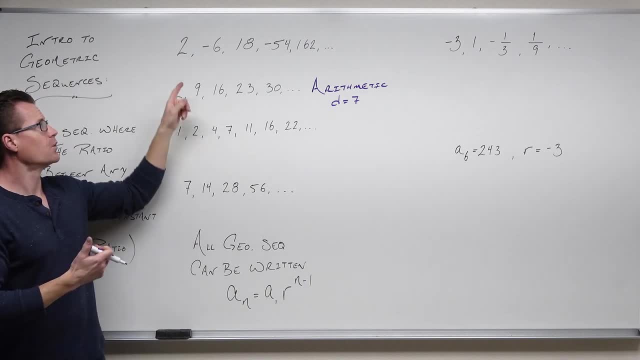 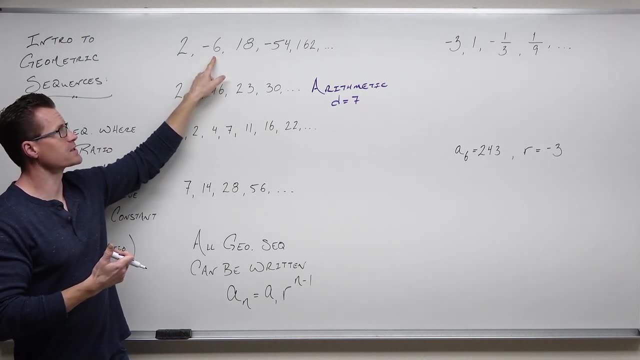 We can think of it one of two ways. Sure, you could think: what do I multiply by to get from 2 to negative 6? Will it be negative 3? Can I keep doing that? Negative 6 times negative 3? Well, that would be positive 18.. Negative times: negative is a positive. 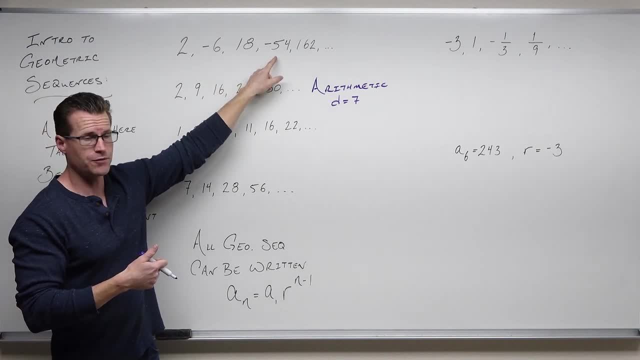 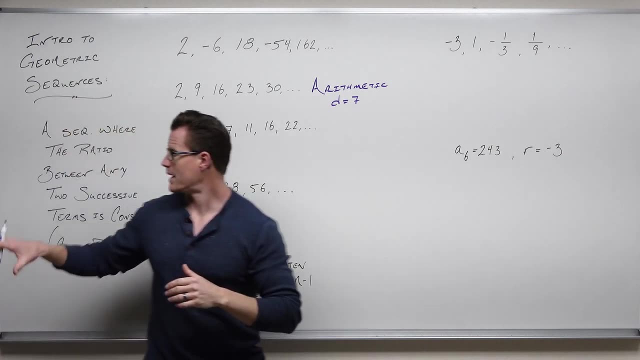 18 times negative 3?? Well, that's negative 54.. Times negative 3, that's 162.. That is what's happening. This is definitely a geometric sequence, but you can also think about it this way If you take any two successive terms and divide them. 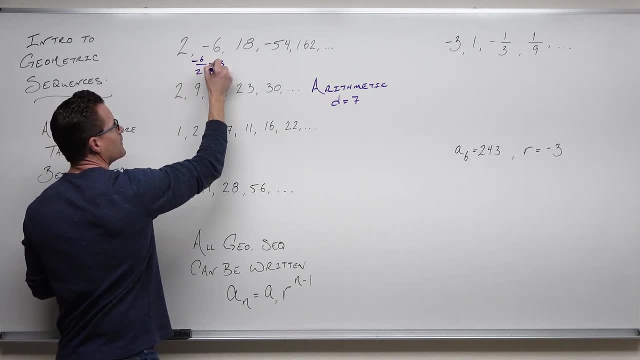 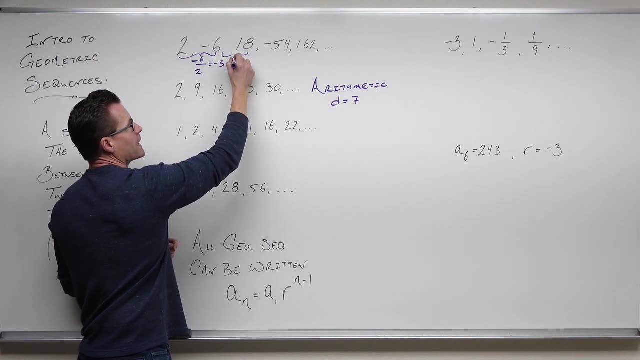 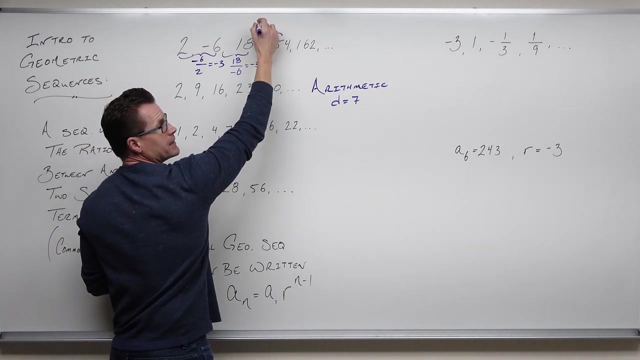 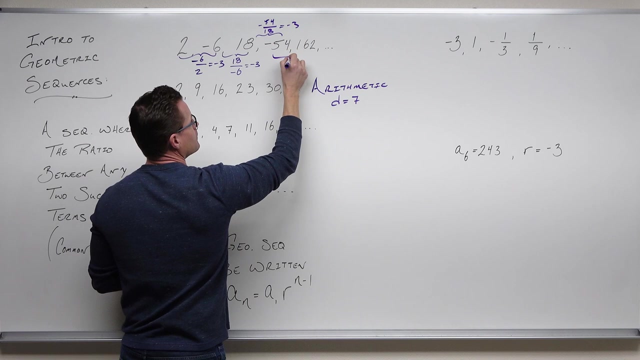 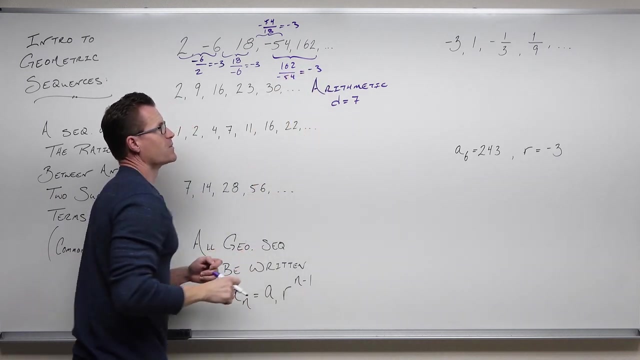 you get negative 6 times negative 3.. So negative 6 divided by positive 2, or 18 divided by negative 6, or negative 54 divided by 18, or 162 divided by negative 54. In each case we get the same number, The number that you get by dividing. 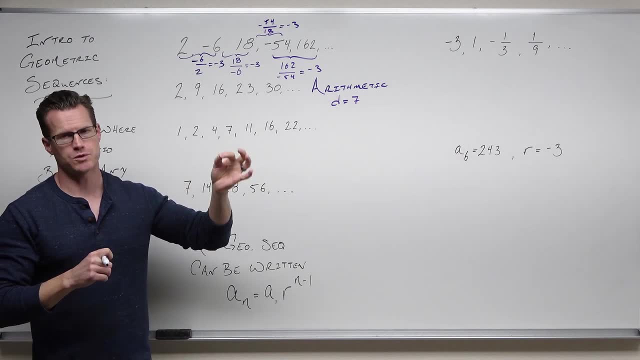 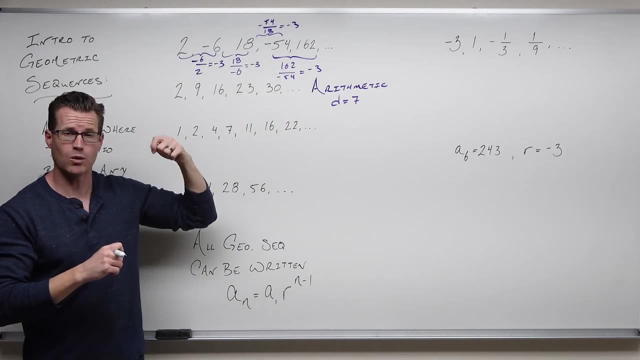 is the same. that common ratio is the same number that you are actually multiplying to get from term to term to term. So this is definitely geometric because we have the same exact ratio between any two successive terms, meaning you are multiplying that same number. 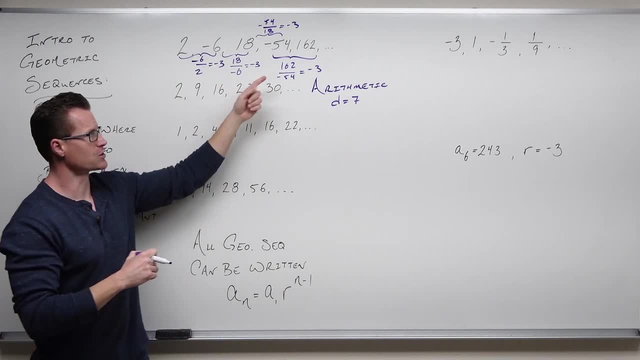 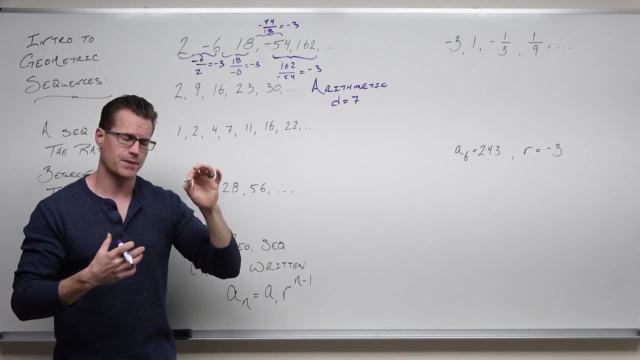 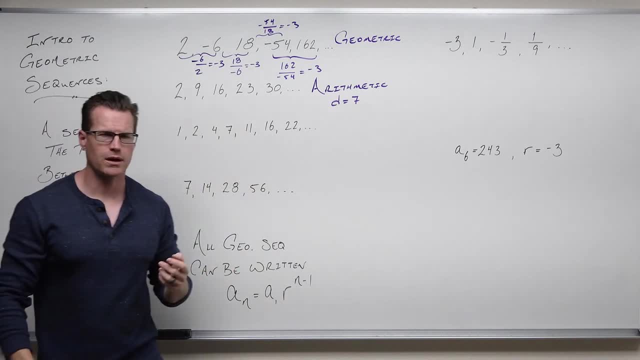 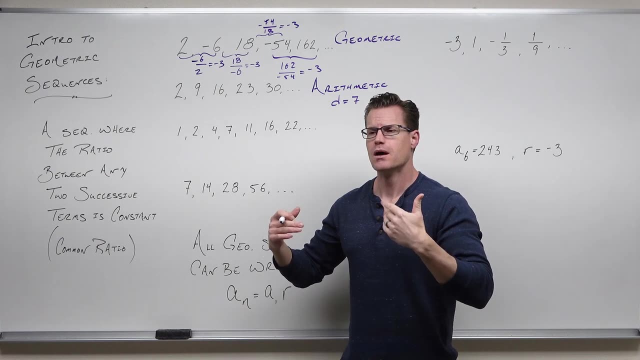 The common ratio is called r. So when we hear that word- that common ratio, common difference was d, It was a d because it was a difference and this term we're actually adding from term to term to term: The common ratio is called r for ratio. 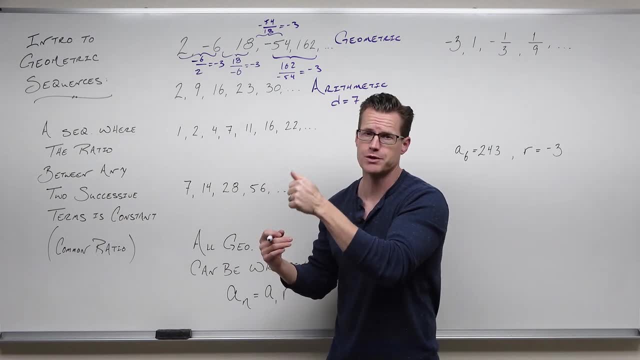 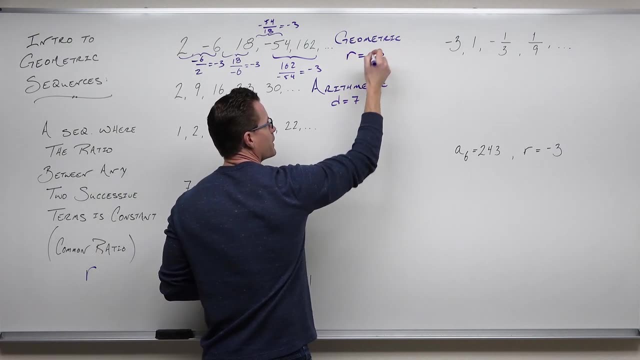 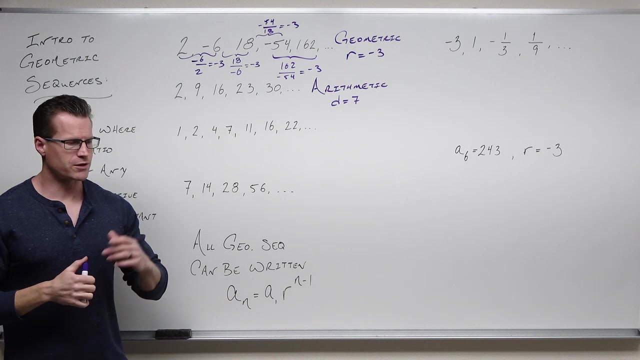 and it stands for the number you're multiplying in a geometric sequence, from term to term to term, The common ratio is d. In our case, it's just negative 3.. That's really the difference between arithmetic and geometric Arithmetic. you're just adding whatever number you're adding. 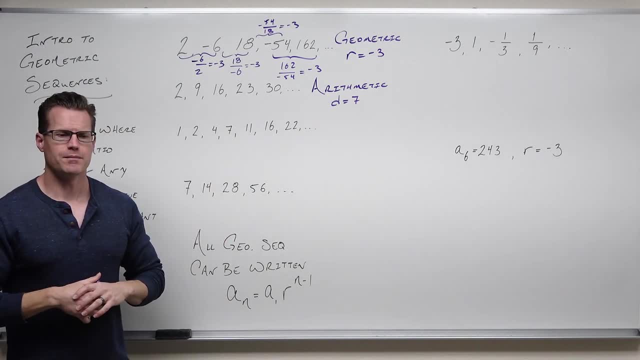 over and, over and over again. That's d. That's your common difference Geometric. you're just multiplying. So whatever number you're multiplying by over and over, and over and over again to get that sequence, that's your common ratio. That's r. You, of course, can find them by subtracting. 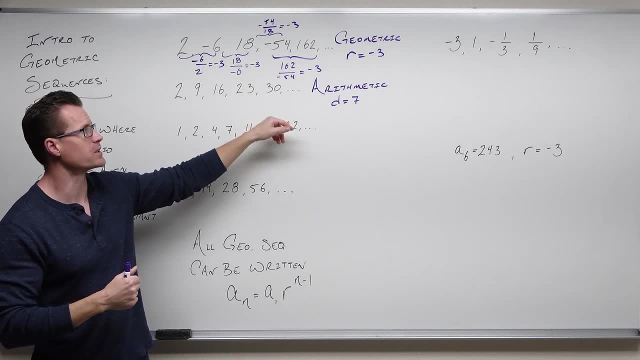 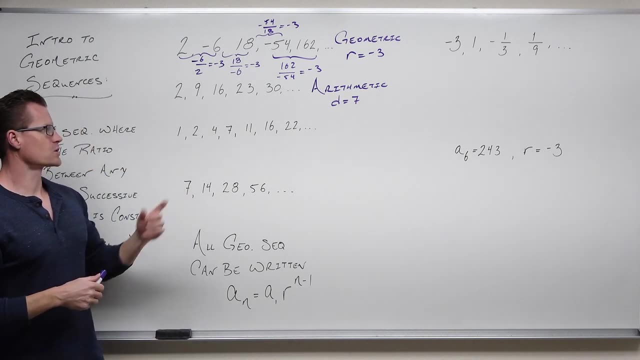 two successive terms, and it's the same for all of them. You have an arithmetic sequence. Or dividing two successive terms, it's the same for all of them, every pair. You have a geometric sequence. Now, how about the next one? So 1,, 2,, 4,, 7,, 11,, 16.. Well, 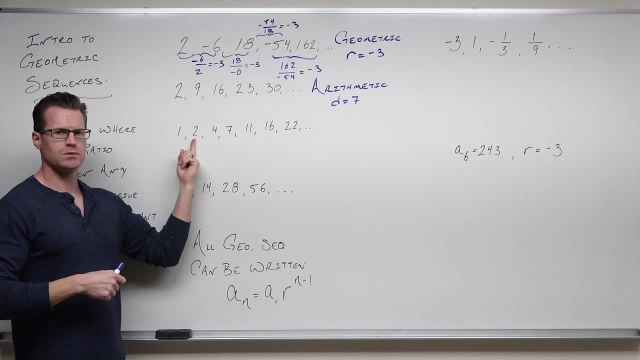 let's try geometric first. In order to get from 1 to 2,, I would multiply by 2.. That's great. In order to get from 2 to 4,, oh, I'd multiply by 2.. That's also great. Maybe this is geometric. 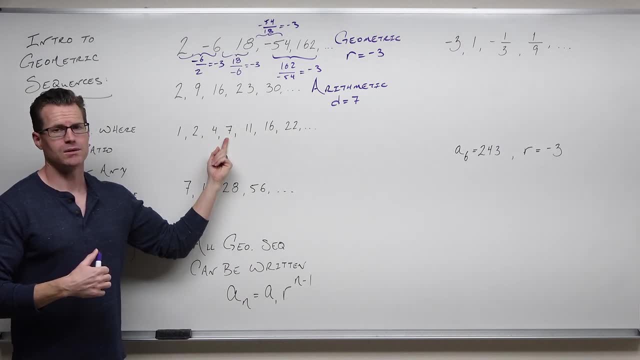 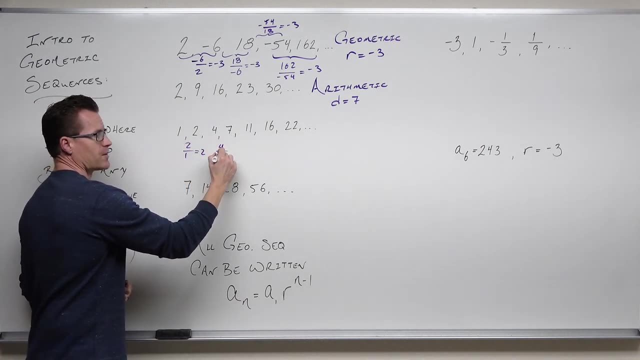 In order to get from 4 to 7, I multiply by 2? No, So even though the first two terms, if I were to divide them, 2 divided by 1 is 2, and 4 divided by 2 is 2.. But 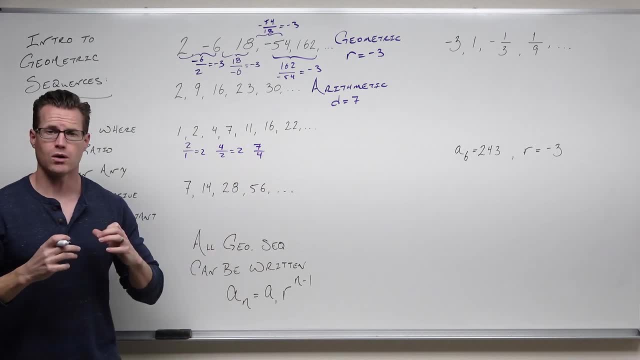 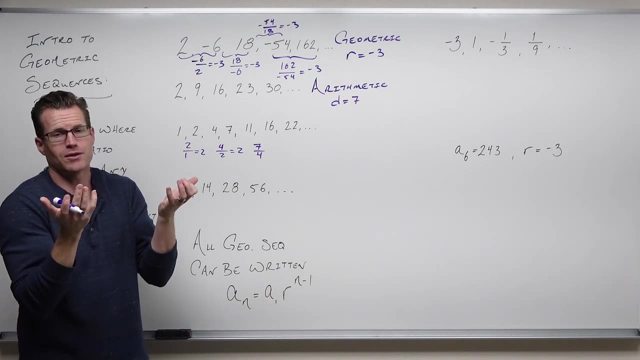 7 divided by 4 is not 2.. And in order for this to be called a certain type of sequence, you can't say like, oh, it's geometric for a little while and then arithmetic for a little while and then I don't know for a little while. That doesn't really work, So it has. 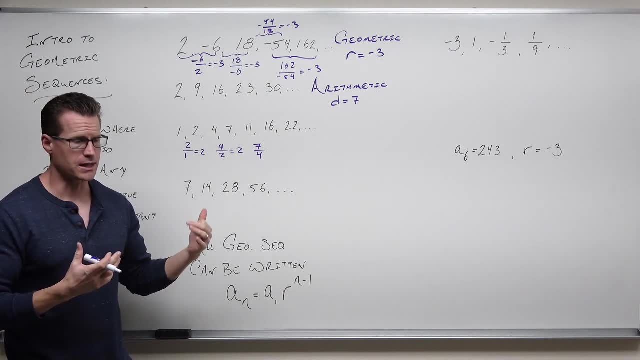 to maintain the same exact pattern, if you're going to call it one of these things. So this common ratio would be well, the a ratio would be 2 and 2, and then not 2. This fails to be geometric, because I'm not multiplying by the same number to get from term. 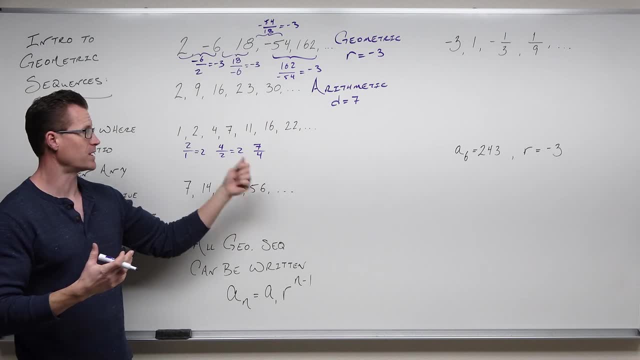 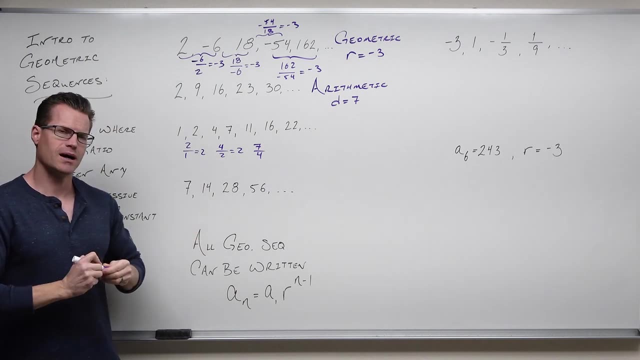 to term to term. I'm not actually multiplying at all to get from term to term to term It. It looks like it may be times two times two times, but that right there starts failing it. This is not geometric, So maybe we try arithmetic and go all right, well, let's try to add. 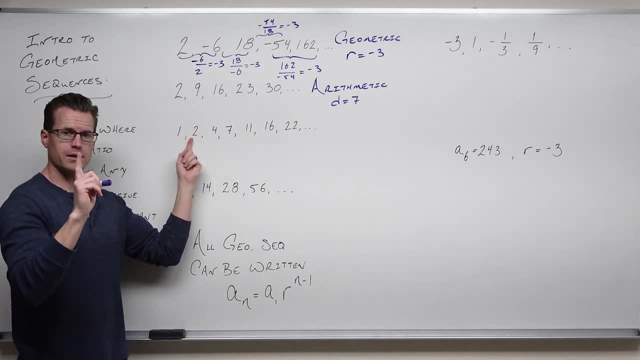 So if I was adding from here to here, I would add one. From here to here I would add two. That already fails, because a common difference for arithmetic says I should be able to take two minus one and four minus two and seven minus four and get the same thing. 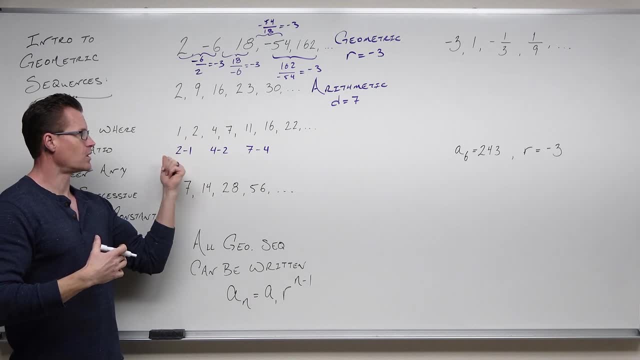 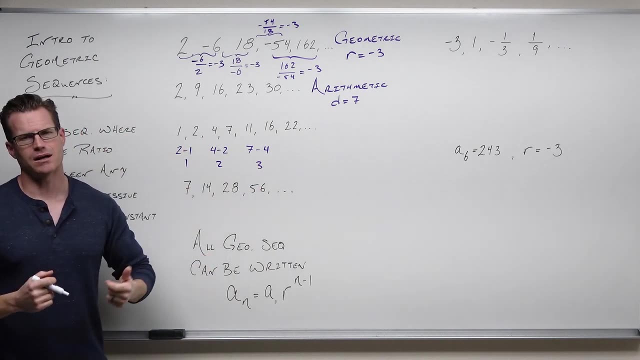 That's what a common difference would do for arithmetic. That was the last video. So two minus one is one, four minus two is two. seven minus four is three. Well, wait a minute. That's not common. That's not the same number being added to go from term to term to term. 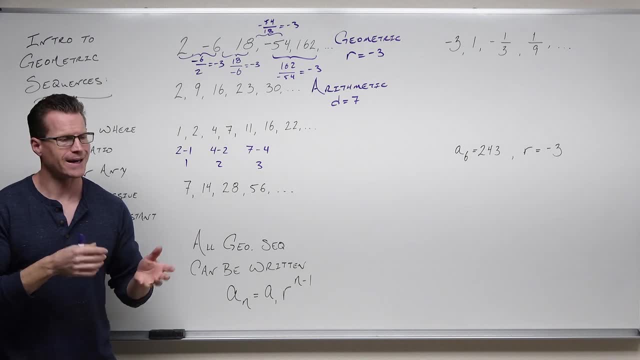 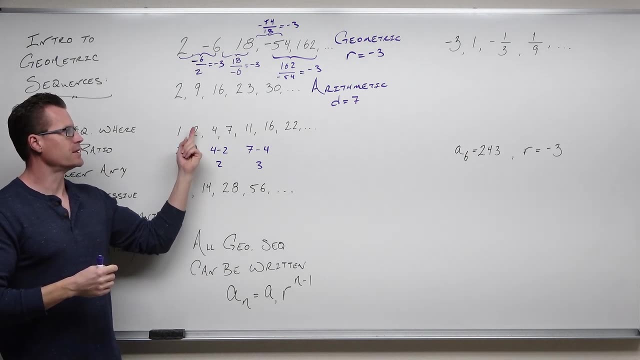 In fact there is a pattern here, but it's not geometric, It's not arithmetic. We've taken geometric off the board. This proves it's not arithmetic. The pattern is: you'd add one, then two, then three, then four, then five, then six. 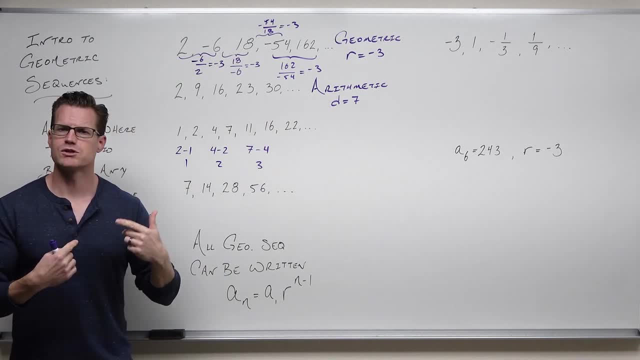 Probably you're going to add seven, next Then eight, then nine, Then 10.. You're just adding successive integers on that. We could certainly find a sequence for that, but it's not something that we're actually studying by name here. 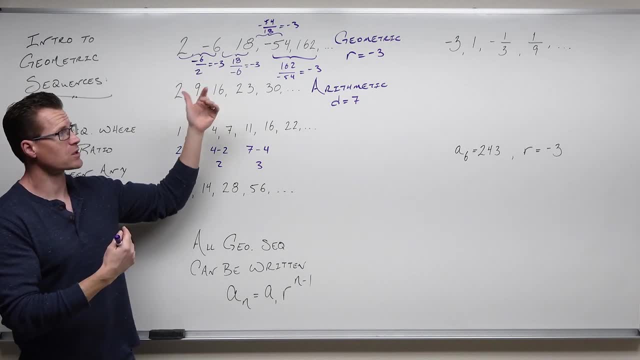 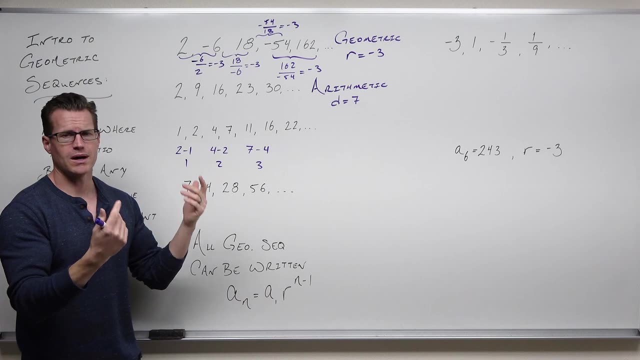 So that's the way we go ahead and determine whether or not something's geometric or arithmetic or neither, You just try them. Just see if you're multiplying the same number, divide two successive terms. just do it for all the pairs. See if you're arithmetic, by adding the same number, just subtract successive terms. see. 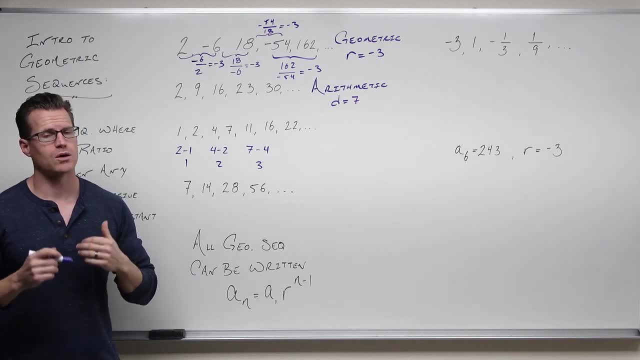 if they're the same Or if you get this. this would be neither arithmetic nor geometric. The next one is a A little bit easier than what we've done so far. Hopefully you can look at this and just say: well, I'm fairly certain. 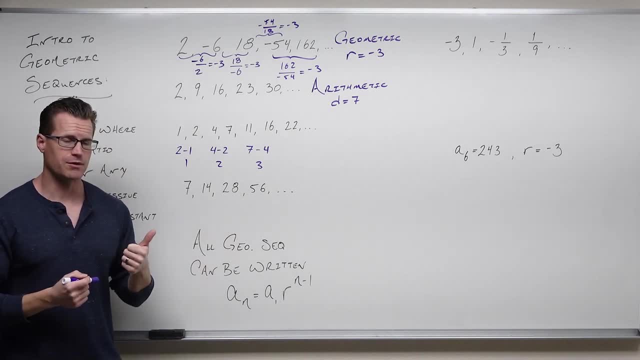 I know what that's going to be because we have the starting spot of seven. Now think how you get to 14 and think how, from 14 to 28,, 28 to 56, are you adding the same number every time? seven plus seven gives us 14 plus seven is not 28.. 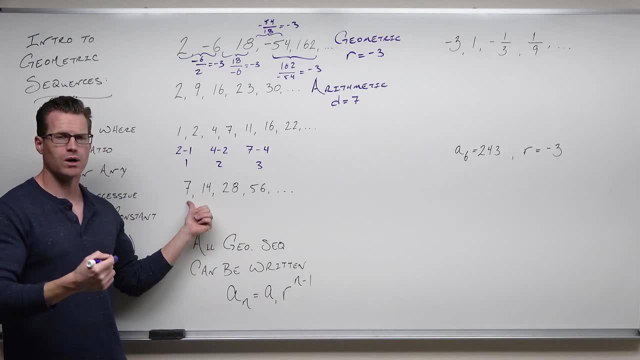 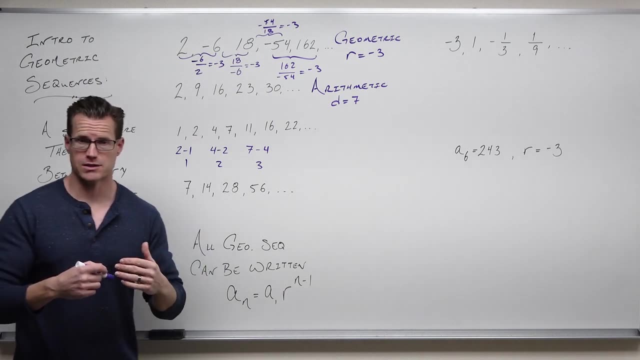 So it's not arithmetic, Let's say geometric: seven times What gives us 14 times two. 14 times two gives us, oh, 28,. 28 times Two gives us 56. If I were to divide this, uh, pair by pair, 14 divided by seven is two, 28 divided by 14. 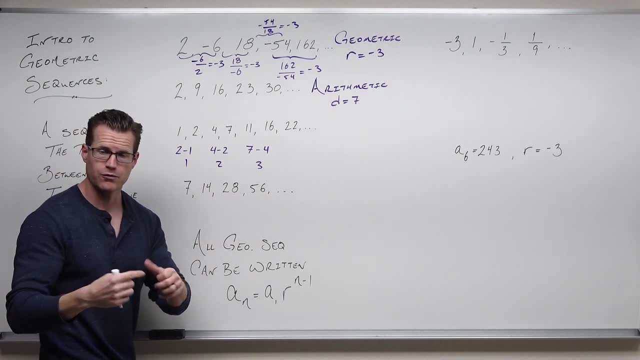 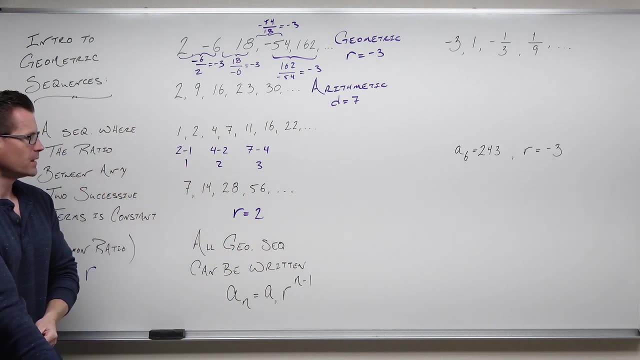 is two. 56 divided by 28 is two. Our common ratio for this geometric sequence is two. Now, what's kind of interesting is that, much like arithmetic sequences did, a geometric sequence has this, this very- uh, repeatable pattern. It's so repeatable. 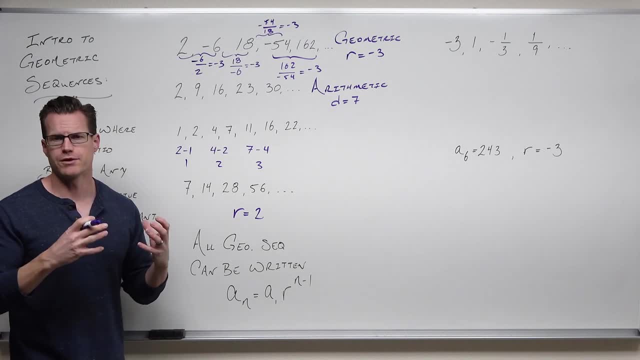 They've been rising formula. So there is a, a model for every geometric sequence. All we need to know is what the first term is and what our common ratio is. Now, just like we did arithmetic sequences, I really want you to see why there's an N. 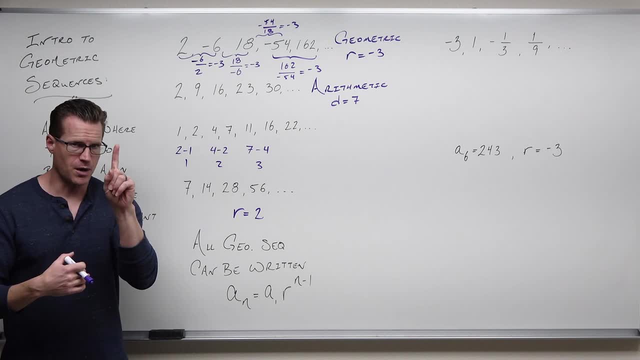 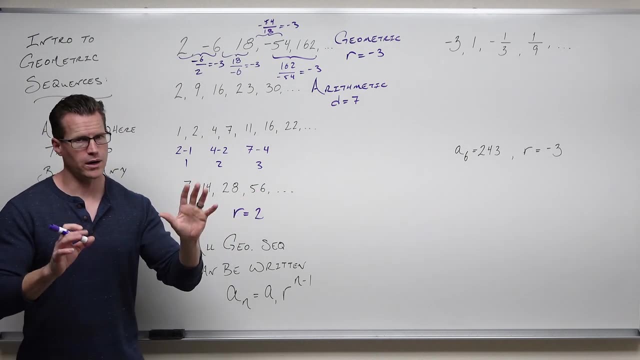 minus one here. So think about this: If you burn up one term by starting somewhere ace of one, then how do you get to your hundredth term? Well, if this is where you start and this is how many times you have to multiply. 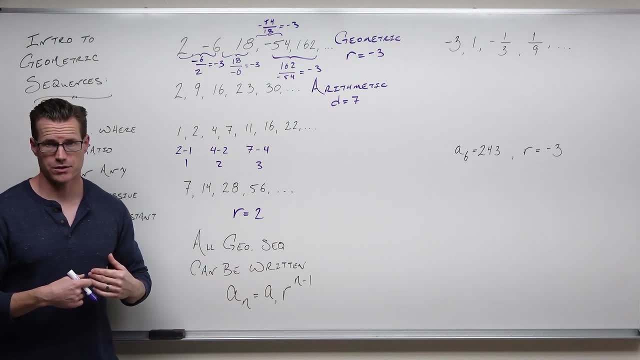 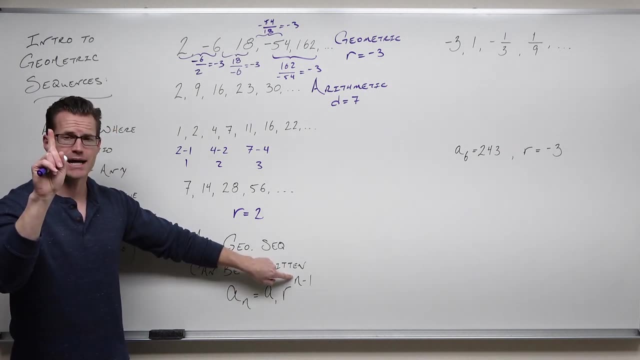 To get to whatever term you want. then let's say I wanted to get to the hundredth term. If I want to get to the hundredth term, I start somewhere. That's one term. I would need to multiply by 99 hours to get to the hundredth term. 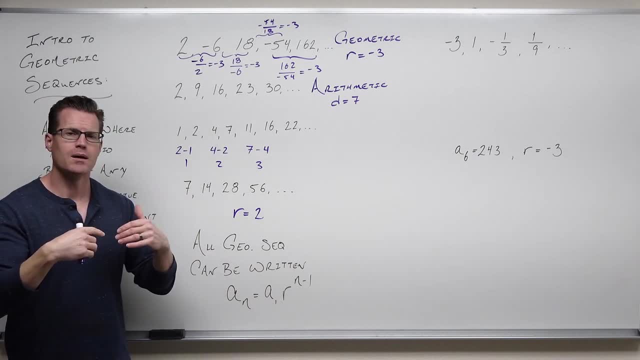 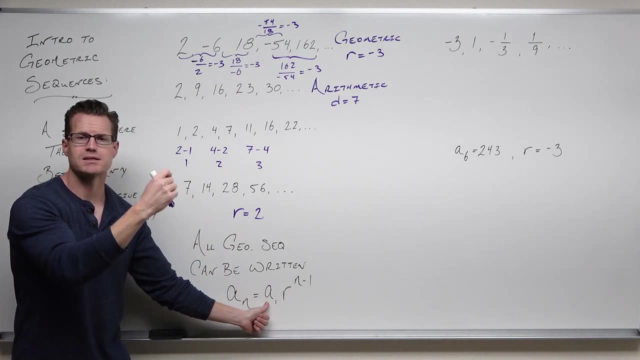 I'm going to say that one more time, in just a slightly different way, by taking up one value by a starting number in order to get to whatever term you need. It's one less, uh, one less iteration of multiplication than the index. index you're. 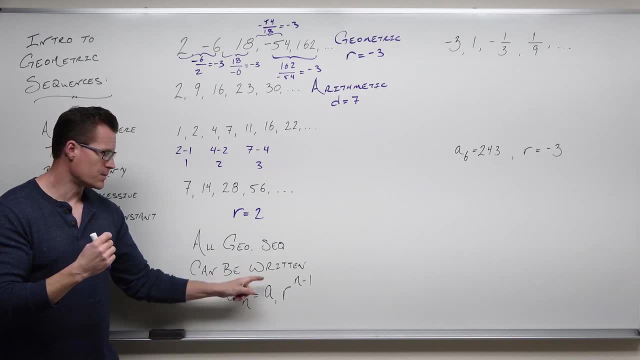 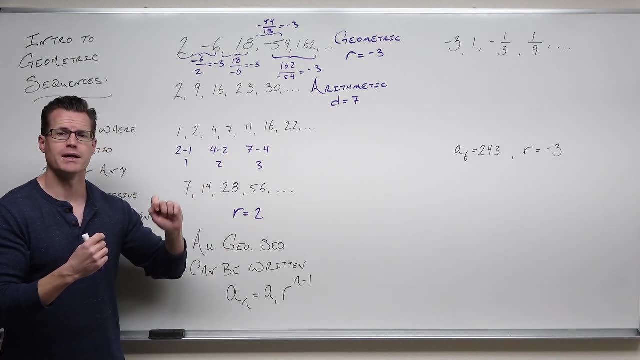 trying to find. So. so again for the hundredth term, I'm using one as my starting term and I need to multiply once to get the second term, twice to get to the third term. on 99 times you the hundredth term. 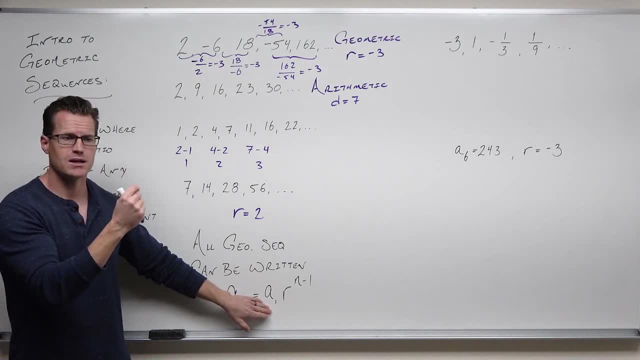 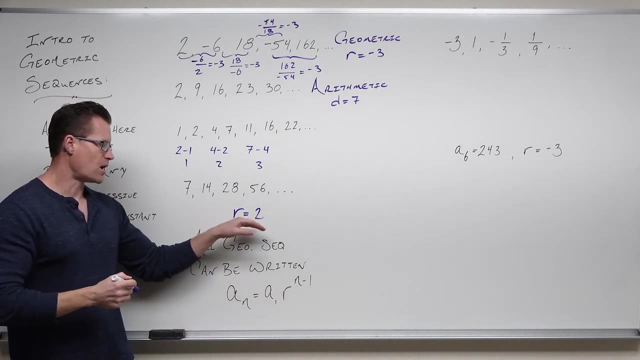 This is losing one of those, It's it's taken away one um necessary multiplication because you're starting with one of those terms. So we would say, all right if I know that my common ratio is two and my starting value. 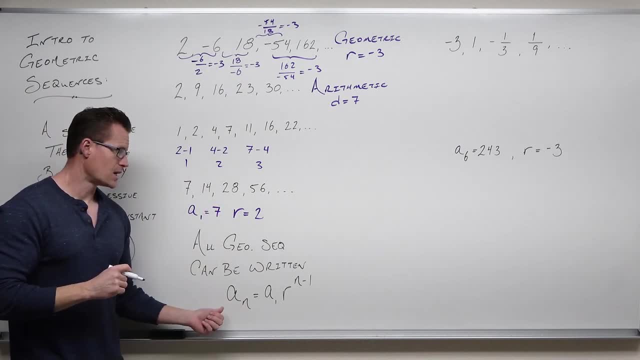 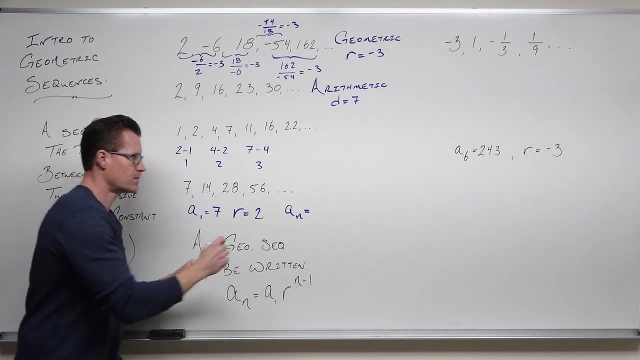 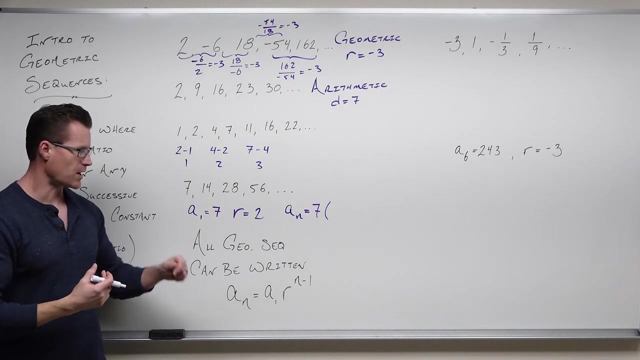 is seven, then I can easily Right This. in terms of the geometric sequence, I can say that this sequence is: take your starting value. You don't necessarily need parentheses, but you're going to see it a lot, especially with fractions. 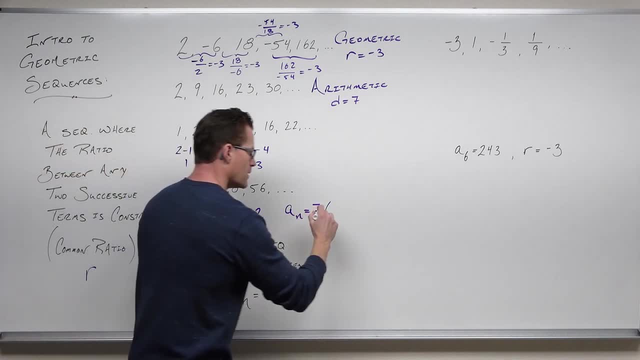 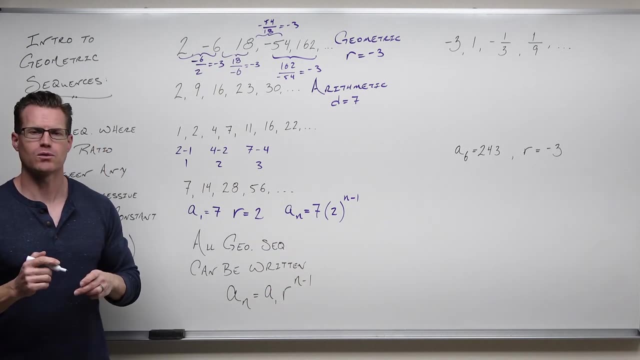 Take your common ratio. That's the number you're multiplying over and over and over again to the end minus one. Do not multiply that and give me 14,. please break an order of operations. You can't do it Now. does it work? 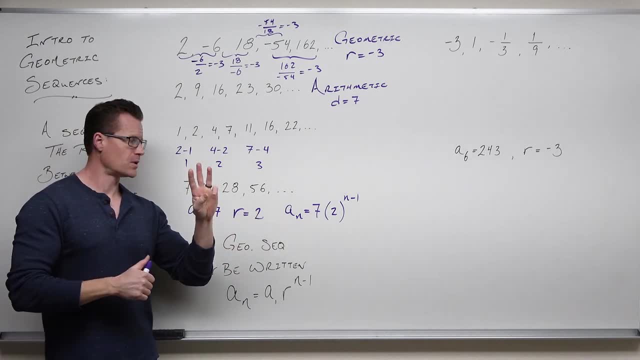 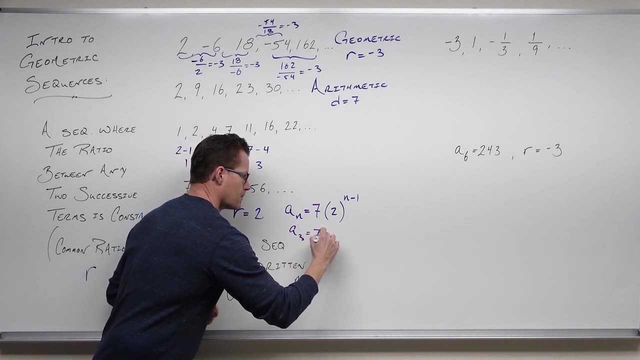 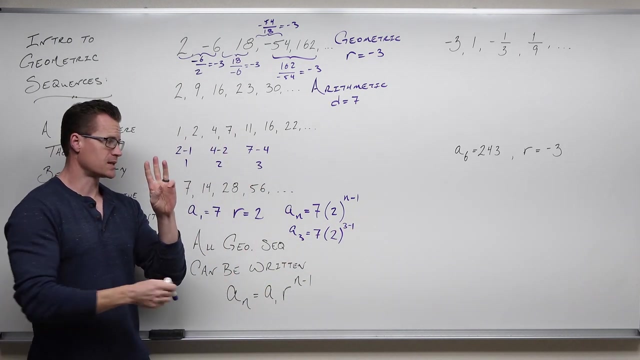 If I wanted to find The third term, check this out. If I want to find the third term, these does 28,. but I want to find ACE of three. Think about what that would mean. ACE of three says I would take seven as my starting term. 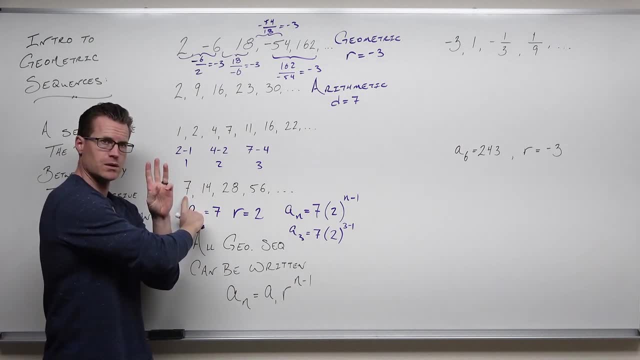 How many times would you have to multiply by two to get to your third term? Well, if this is my starting term, that counts as one. I'd multiply by two, once for 14 and twice for 28.. Not three times. That's why there's a minus one right there. 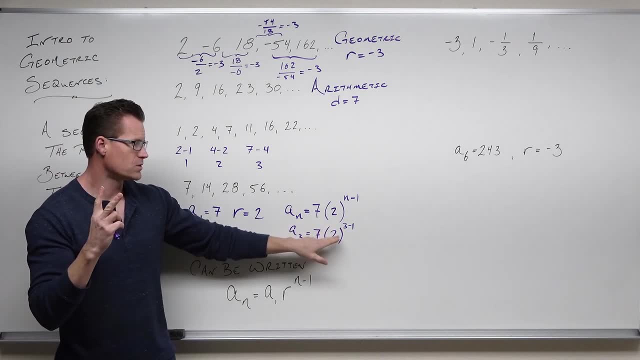 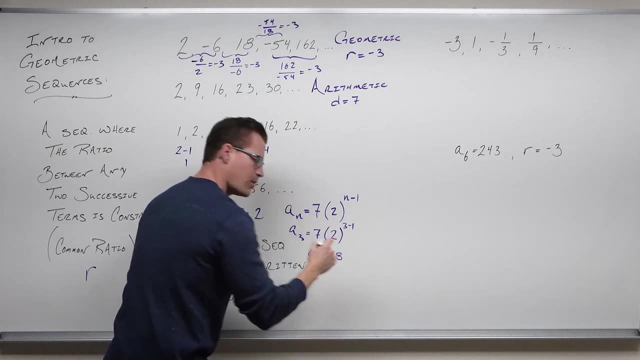 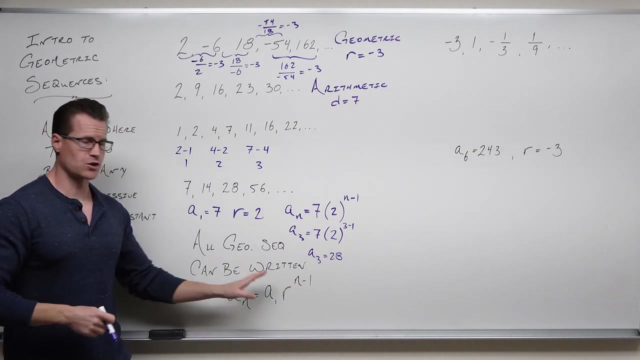 And this would actually work. Three minus one is two to the second powers. four and seven times four would be 28.. I hope I'm making that makes sense to you that you're you're only having to multiply by one less iteration of that common ratio than the term you actually want to find. 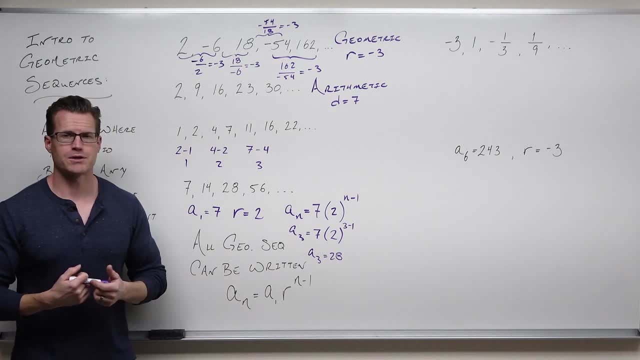 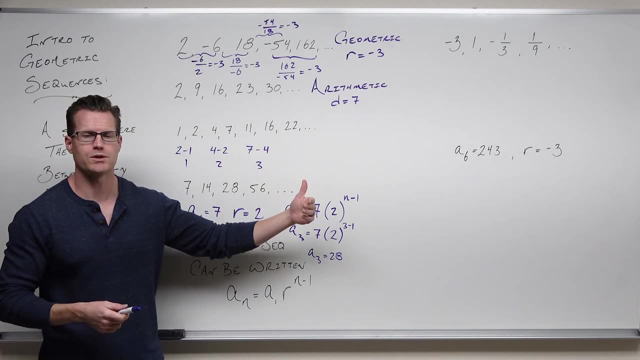 So now we find any term, though. So if I actually find like the 10th term, man, this is really nice, because you wouldn't have to continue This pattern. say, multiply by two, two, two, and then like four more twos or five more twos. 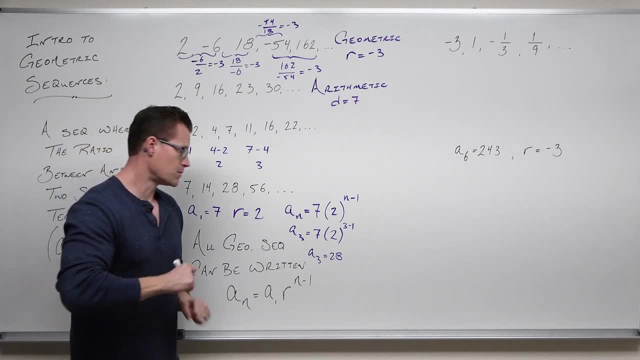 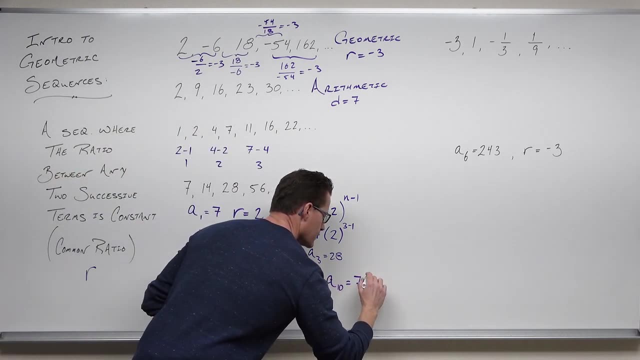 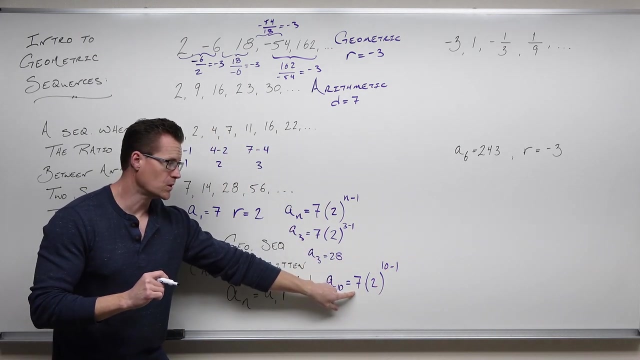 You wouldn't have to do that. All you'd say if you wanted to find the 10th term. We know where we're starting: seven, And if we're starting with seven, we would have to multiply by two, nine times to get to the 10th term. 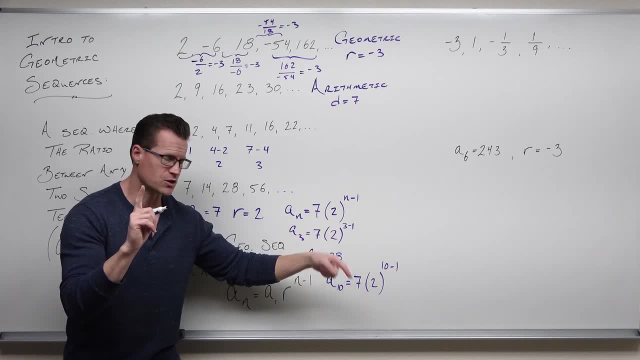 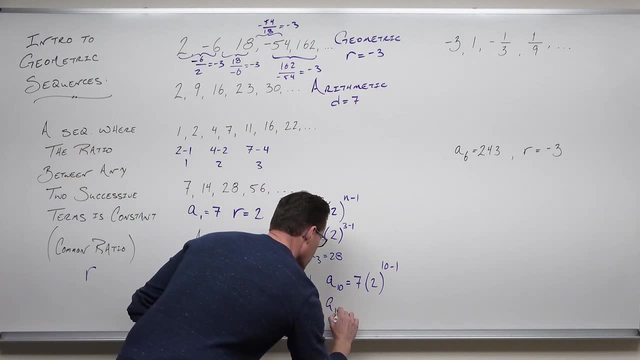 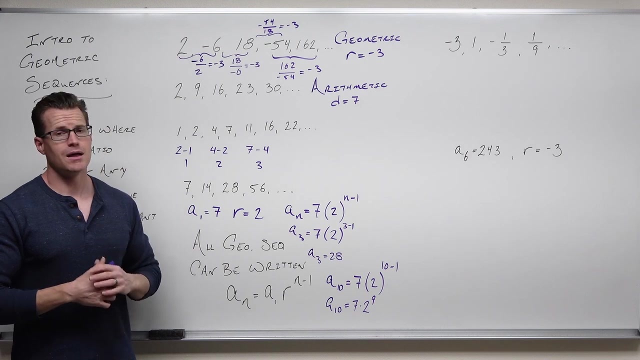 This takes up the first term. I need nine iterations of multiplication. Right Repetitions already get the 10th term, So that would be seven times two to the ninth. So we figure out to the ninth and then multiply by seven. whatever that is, that is your 10th term. 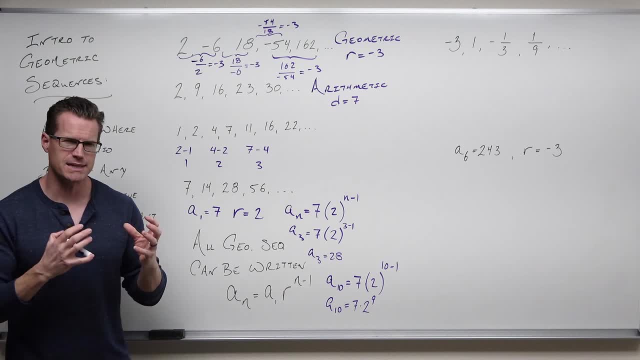 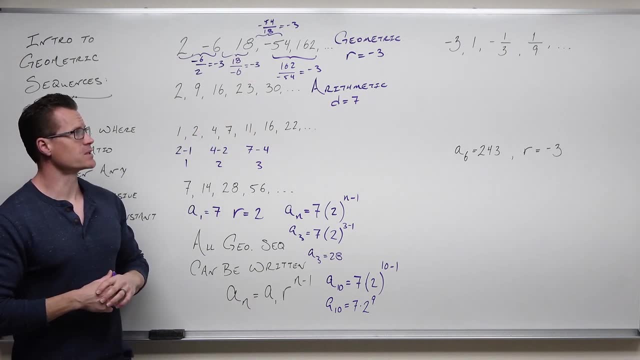 And you can do this with any term that you want to. with the geometric sequence, Very similar idea to arithmetic. We're just multiplying over and over again. Let's go back to this geometric sequence and see if we can write that one. So in order to write any geometric sequence, we need to know where we start. 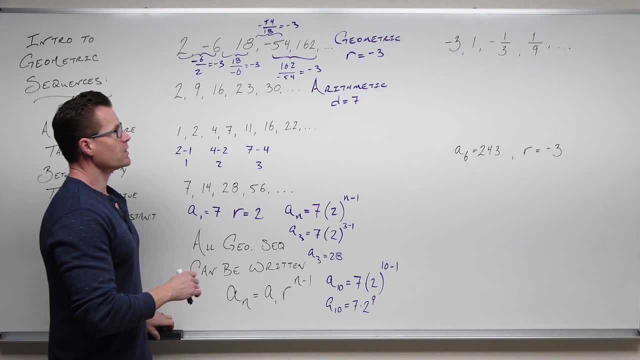 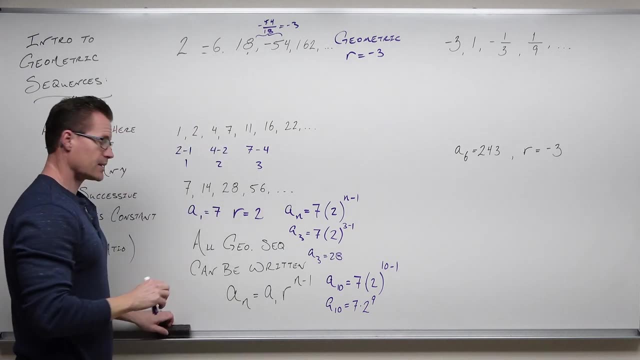 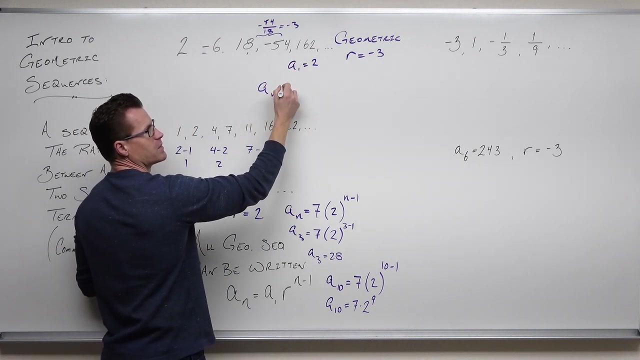 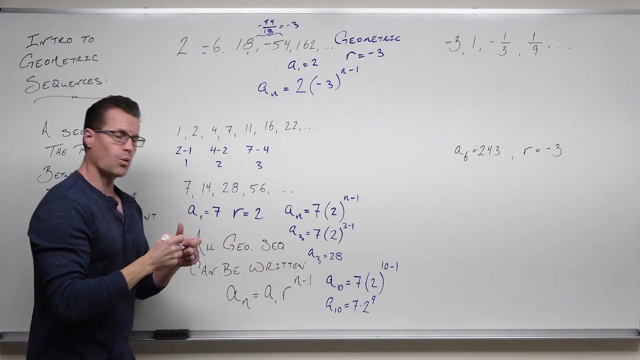 And what our common ratio is. we already found our common ratio. But if we know where we start, if we take a look at that And understand that our starting value, our first term, is two, then our geometric sequence can be modeled by our starting number. times our common ratio to one, less than the nth term. 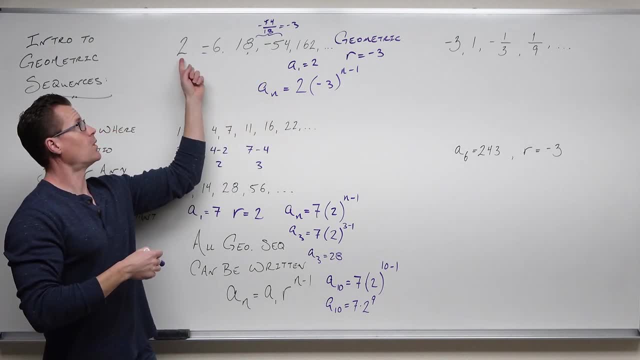 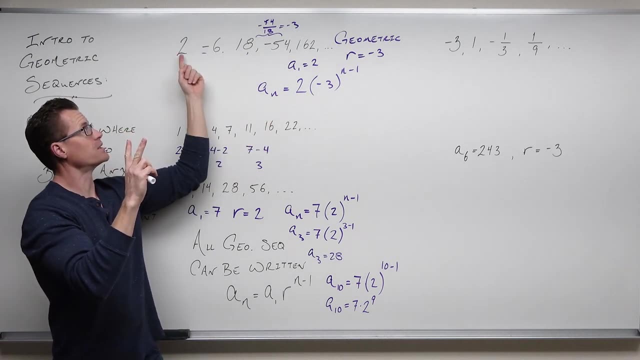 So n minus one, And this actually does work. If I want to find One, two, three, four, fifth term, I'd start at two. I would need to multiply by negative three. Let's see one, two, three, four times. 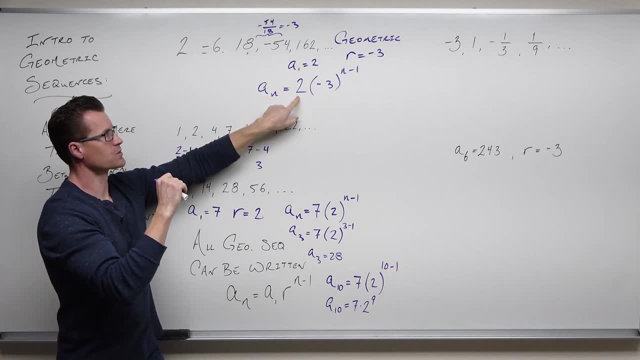 Let's see if that works. Plug in your five certain native two. that counts as one. five minus one is four. native three to the fourth power is positive: 81, 81 times two is 162.. It works just fine. This works very well. 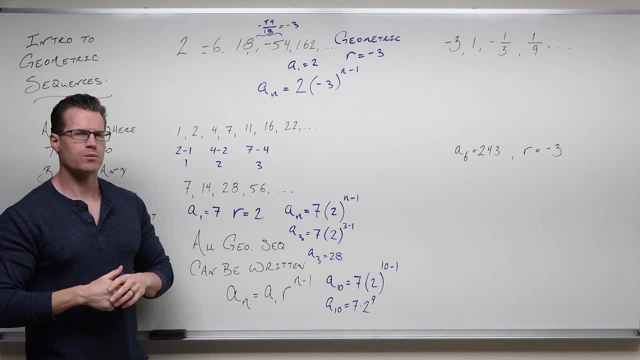 So let's go ahead. We're going to do three more examples: these two and then one more where I give you a Two terms. I'll show you a special way to deal with that, And then, uh, then we're done. 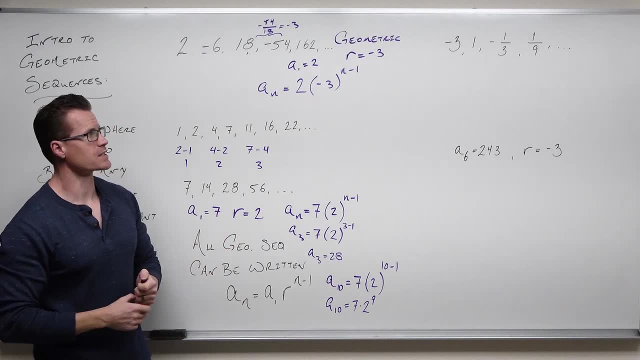 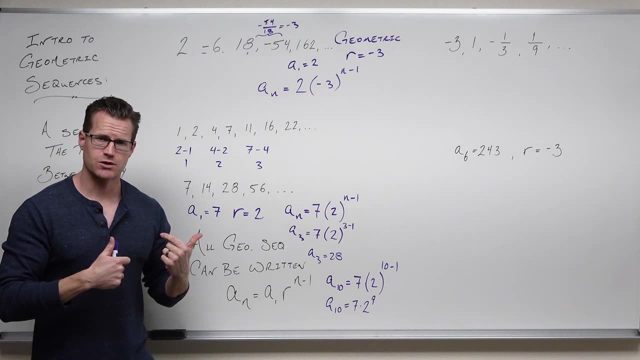 This is all we have to deal with in geometric sequences. Then we'll add them up in our series. So if you were to look at that, how do we know when something is geometric? Well, we can always divide two successive terms or think about what number I'm multiplying over and over again. 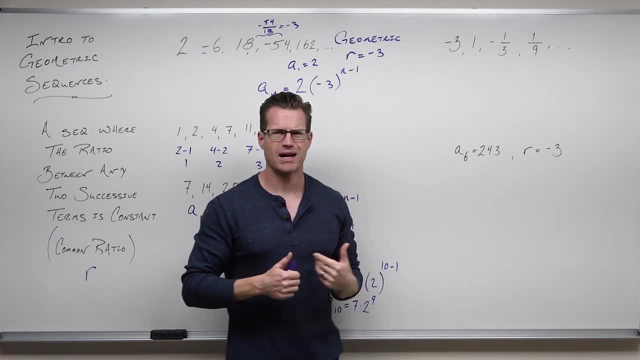 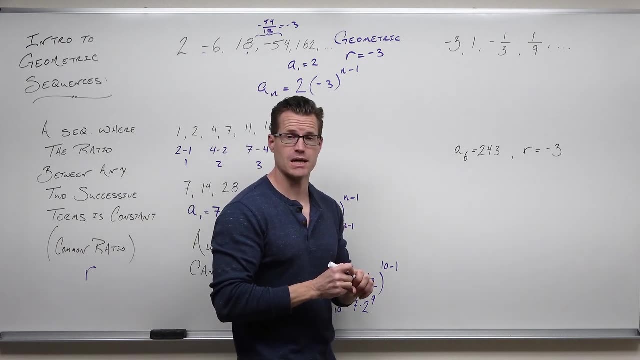 So how do I get from negative three to one? that that might be kind of tricky to think of multiplication, Sometimes it really does benefit us to just divide all of our successive terms and see if it works out in the same ratio. So if I take one divided by three, notice is always that way. 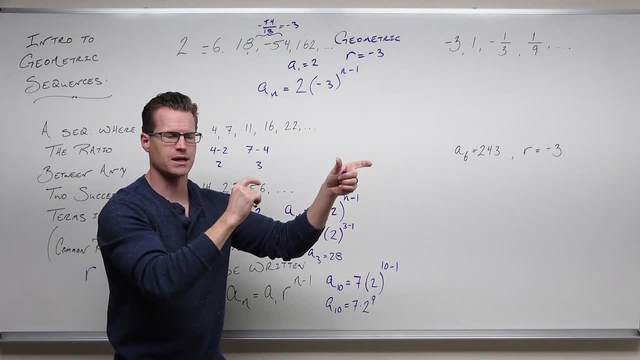 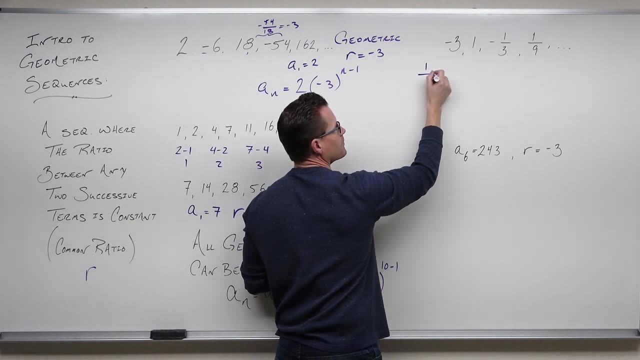 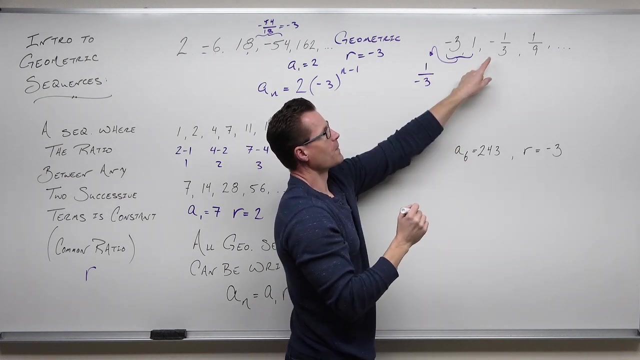 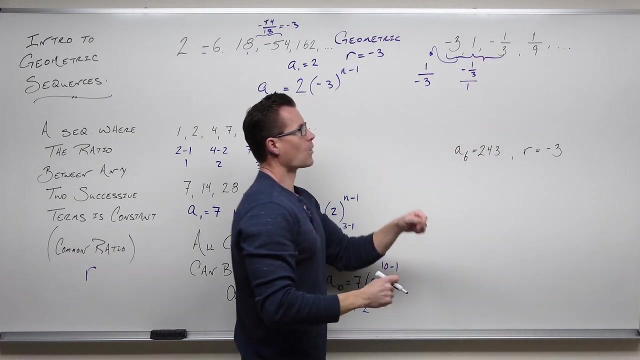 It's always the second term divided by the first, or the third term divided by the second, the next term divided by your current term. So this one divided by that one, one divided by negative three, or negative one third divided by one, or one ninth divided by negative three. 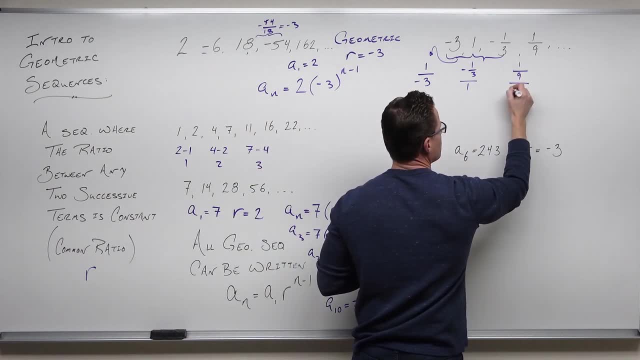 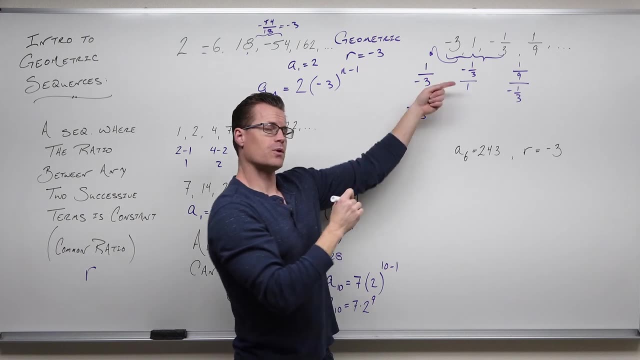 Okay, Okay, Okay, Okay Okay. Negative one third. One divided by negative three. Well, that's negative one third. Negative one third divided by one. Well, something divided by one gives you back that something. That's negative one third. 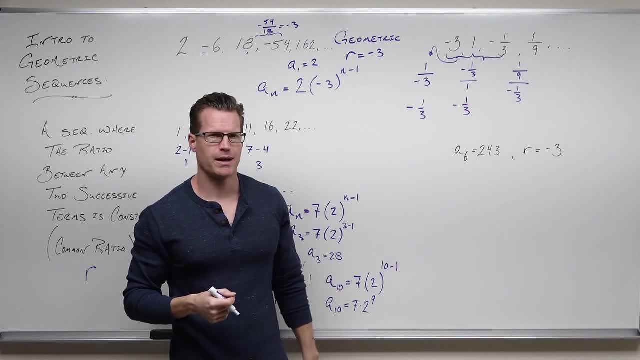 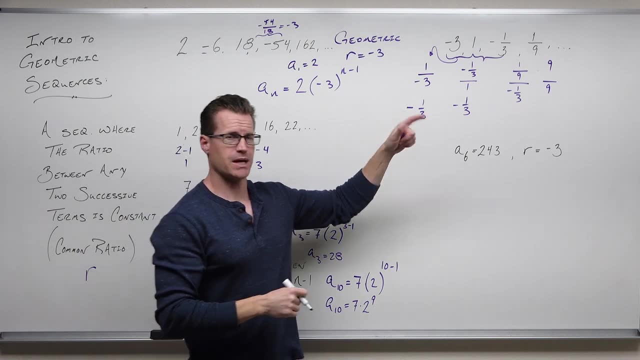 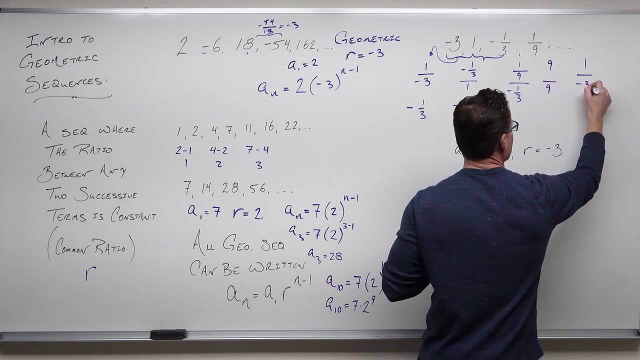 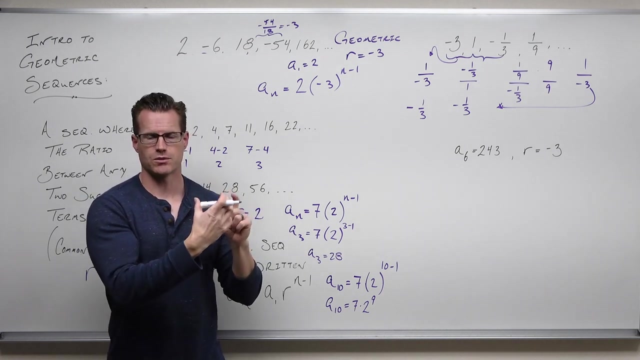 That's looking pretty good. This one we probably want to verify. Maybe multiply by nine As an LCD: One ninth times nine is one Negative. one third times nine is negative, one third Negative three, And we get negative three, negative one third for every single time. we compare two successive terms. 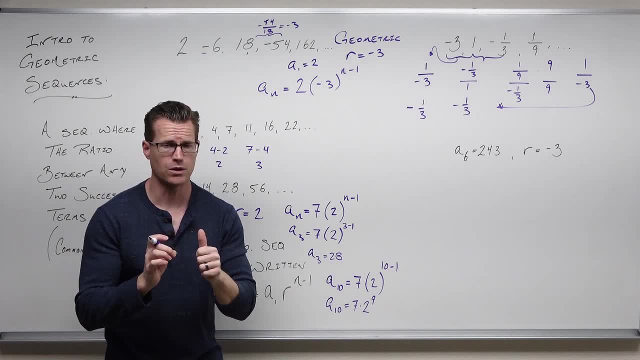 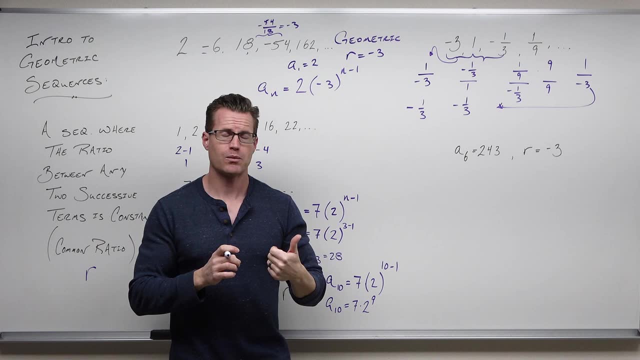 That is a common ratio. So that's the reason why we do in this order. We want to make sure that when we divide we're actually getting the common ratio. We don't want to divide negative three by one and negative three, because that would make us assume that R is negative three. 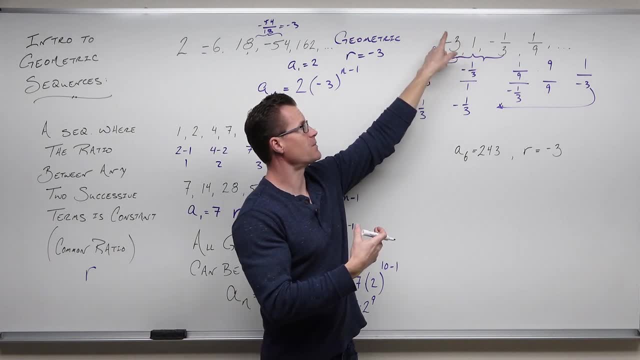 It's not. If we divide in order I've just told you, take the second divided by the first, the third divided by the second, the fourth divided by third, It always gets negative three. So we need to give you out your common ratio and you have to change it. 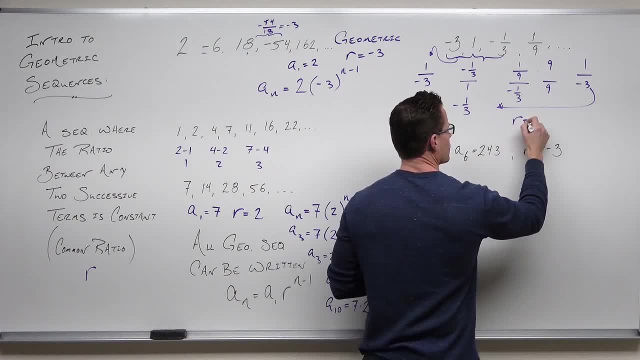 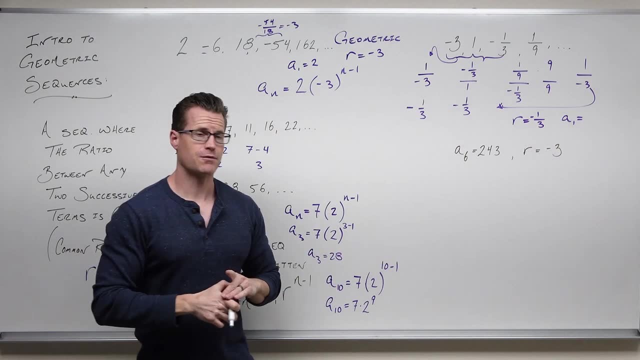 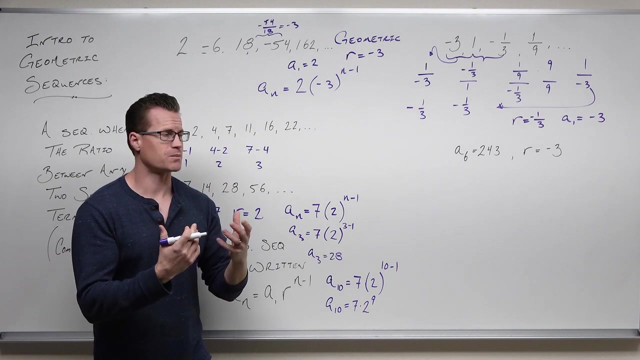 Our common ratio is negative one third, With our first term of negative three. We can easily go ahead and model this with a geometric sequence. We know it's geometric because it gives us a starting spot and it gives us the same exact multiplication term by term of negative one third. 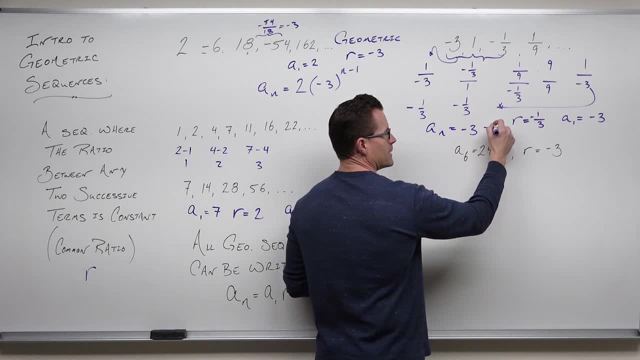 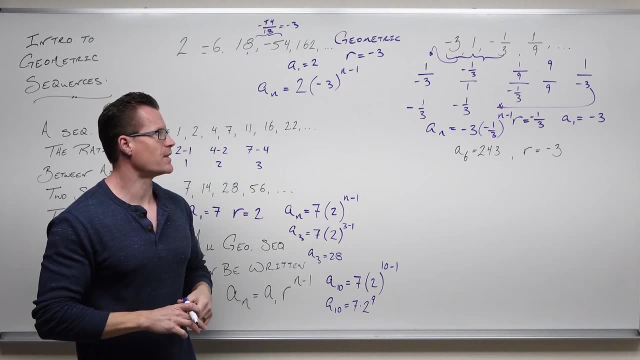 So our geometric sequence says: you start at negative three, You start at negative three three. you'd have negative one-third to the n minus one, and that's perfectly appropriate. There are a couple ways you can manipulate that, but this is just fine for most of our cases. So 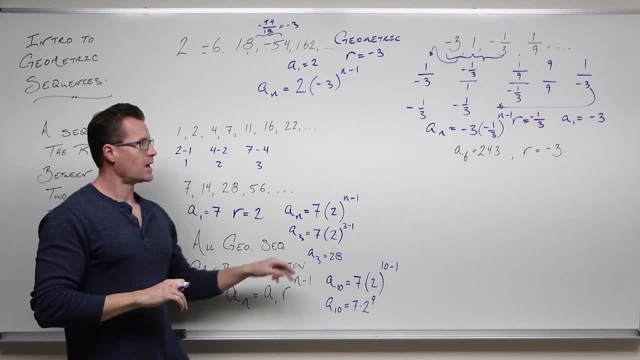 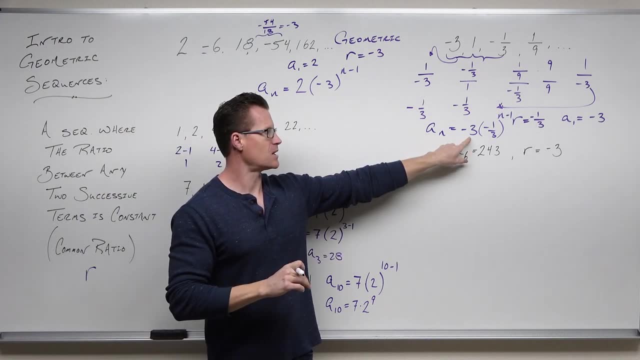 starting number negative three. that's what this says right here. and then your common ratio: negative one-third. we figured that out to the n minus one Again, remember that what this says is: this takes up your starting position, your first term. therefore, you need one less multiplication. 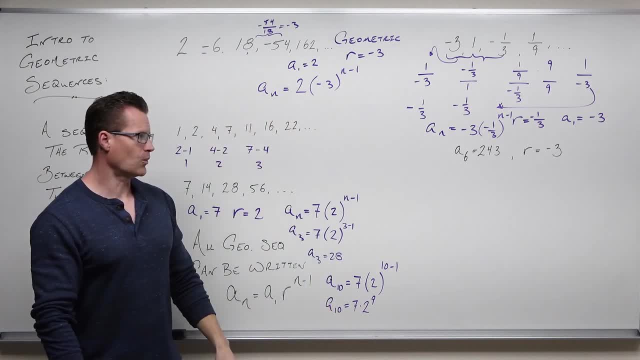 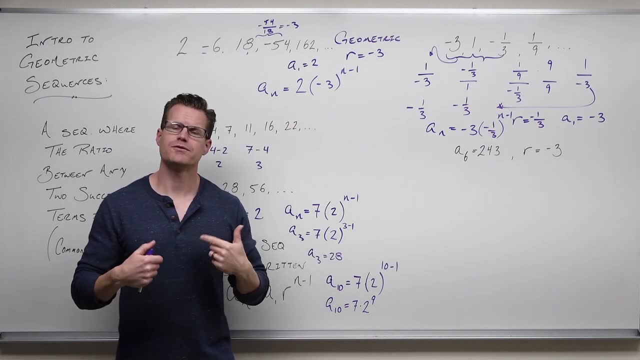 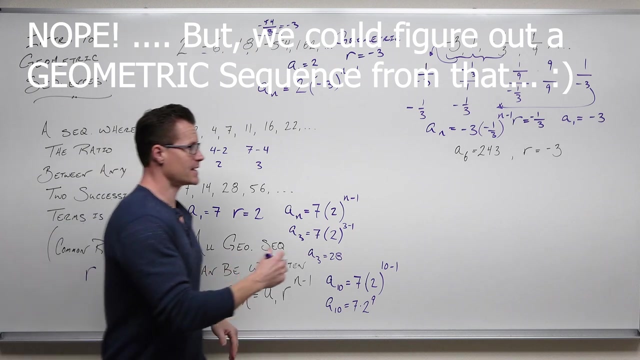 than the term you're trying to reach. Now what happens when they give you some term, but not the starting one, but they do give you the common ratio? Can you figure out an arithmetic sequence from that? It's actually not that hard to do. We just need to remember what this says. So this says: 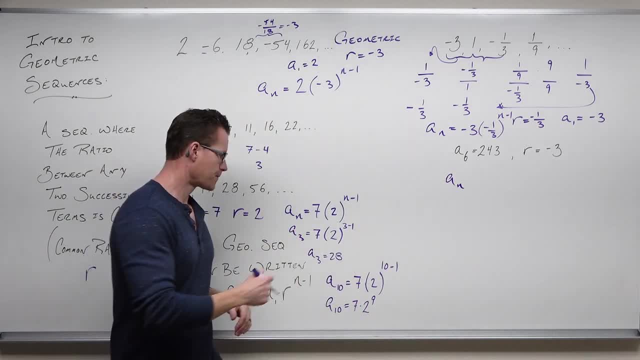 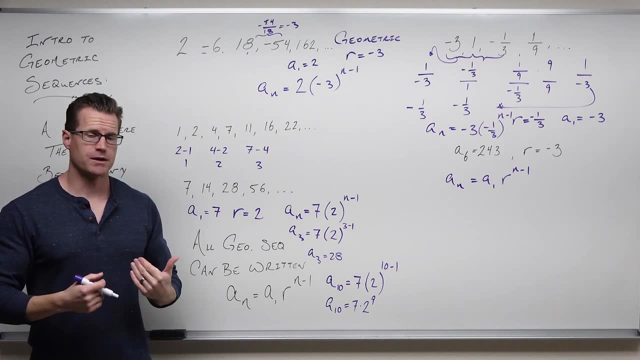 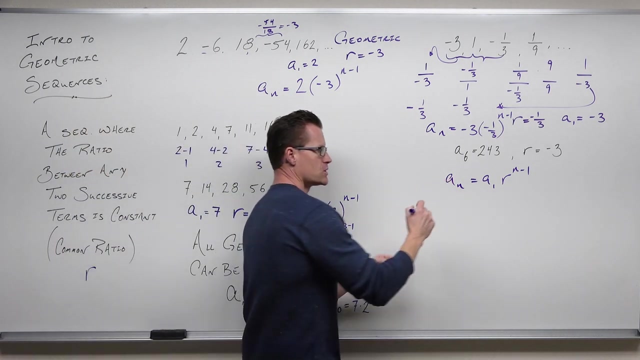 any term that you want is modeled by that sequence. Well, let's plug in the things we know What? What do we know? Well, we know that the sixth term is 243. So if I put 243 for my term that I know, 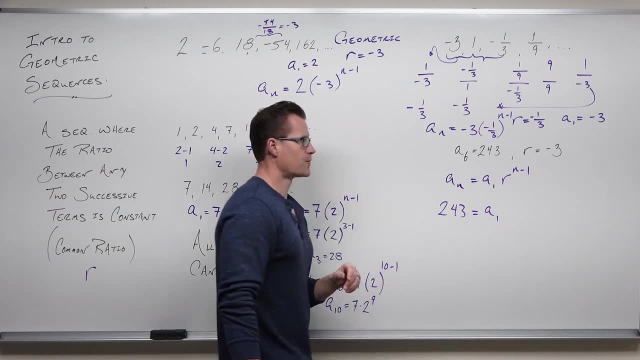 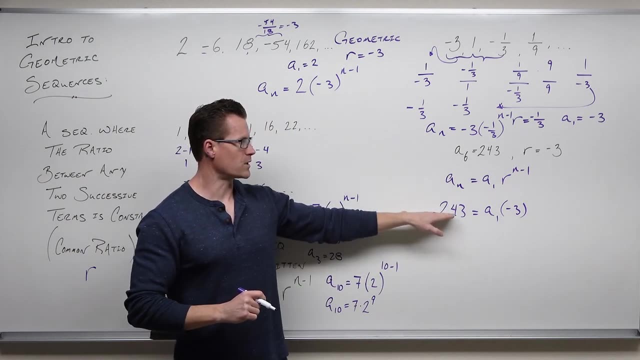 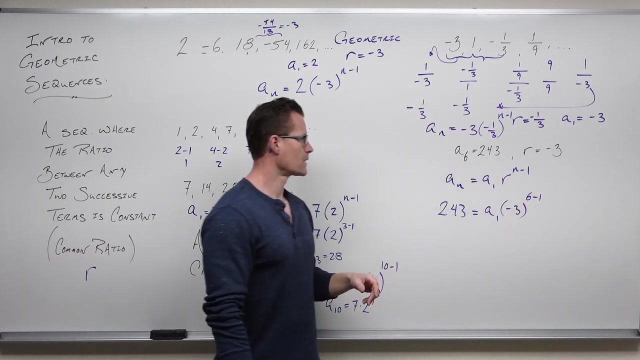 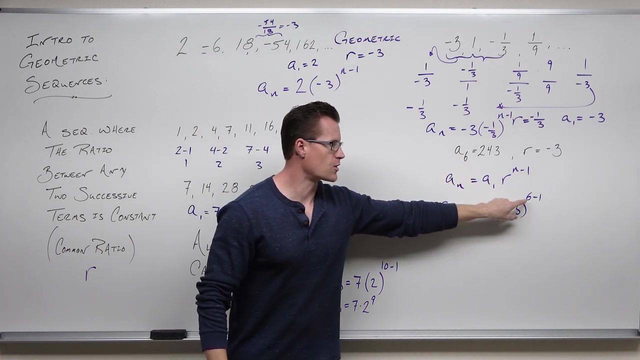 I know that's 243.. While I don't know my first term, I do know my common ratio and I also know that 243 is the sixth term. So my n has to be six. So my term that I know is 243, and that represents the sixth term in that sequence. So let's just fill up the formula. 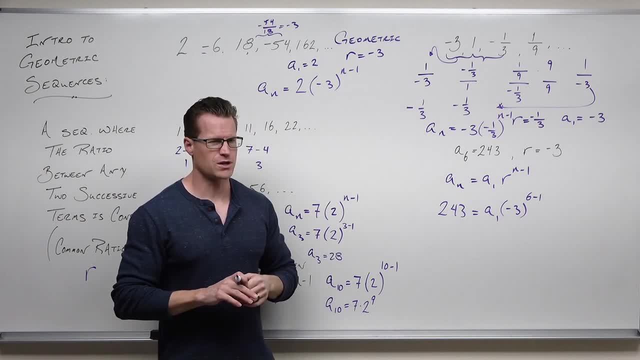 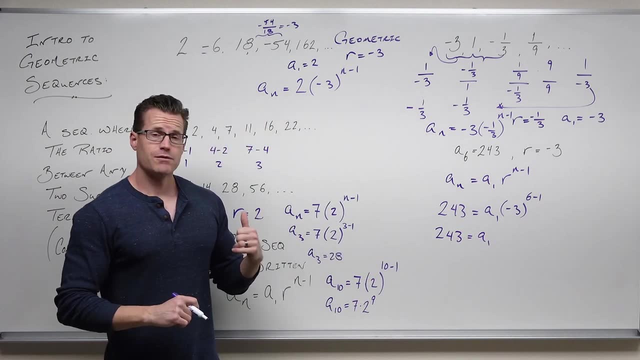 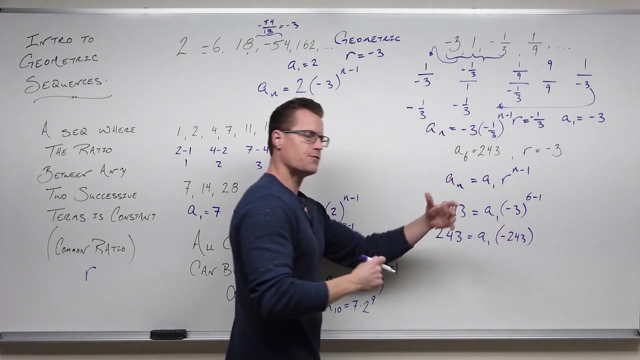 After that you should be able to see that this is pretty nice to solve for r. It's not all that bad. So this is: 243 equals a sub one. Negative three to the fifth power is negative 243. And if you divide both sides by negative 243, you're going to get a sub one is negative one. 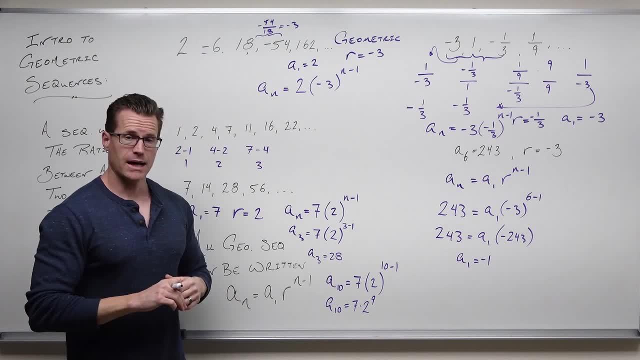 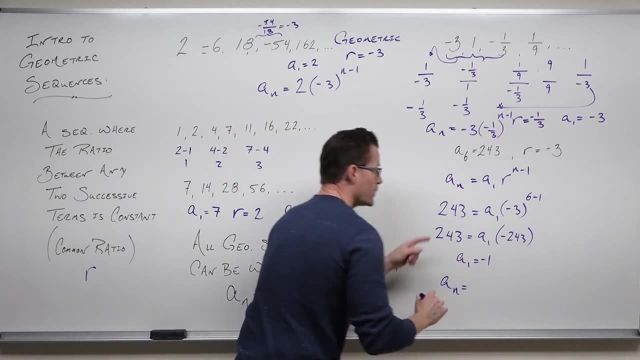 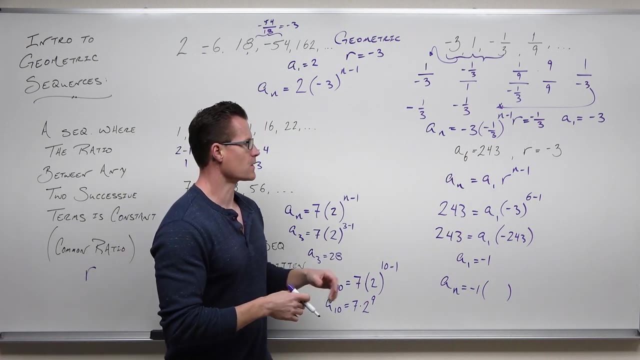 Now this allows you to plug this into this formula. So we now know the general formula for that sequence. We know the first term is negative one. You generally wouldn't want to write the negative one, but I'm showing that to you here. You know your common ratio. 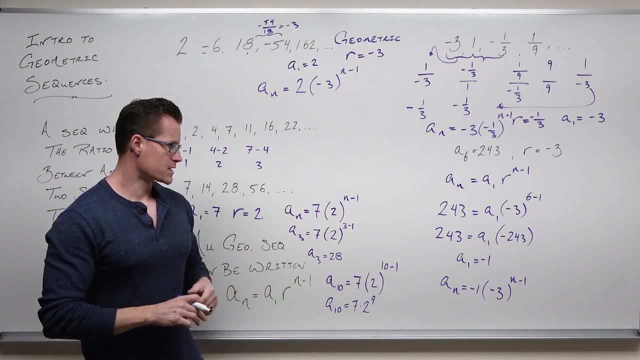 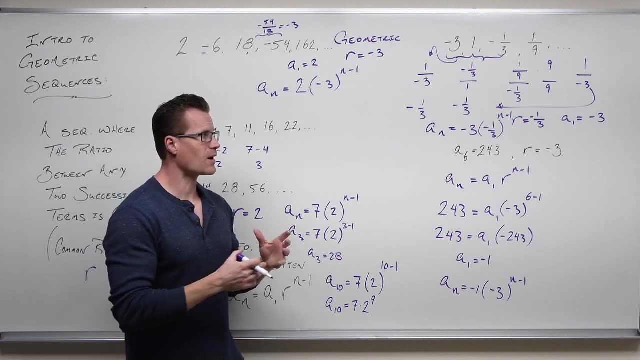 and that would be the form of our sequence. We have our first term and our common ratio to the n minus one power. That's about all there really is to it. You're just trying to figure out from your sequence what your first term is. You need that. 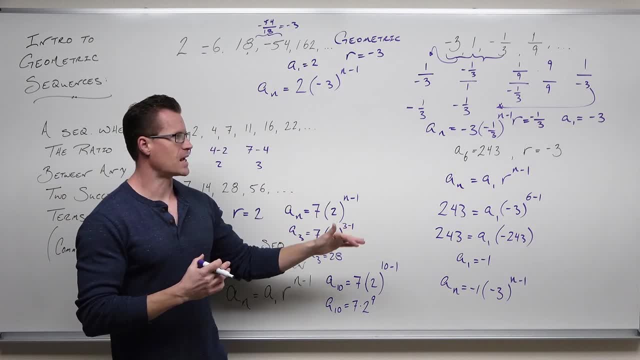 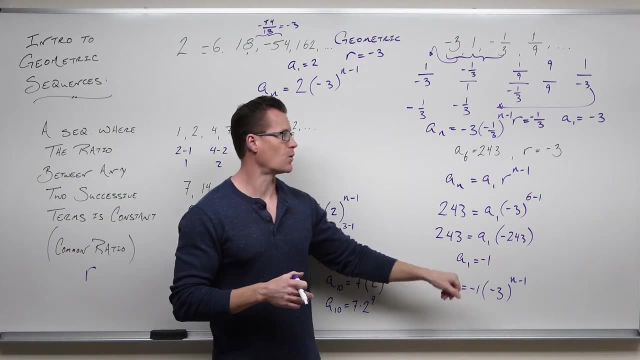 And then you need to know what your common ratio is. From here on all these examples, you should very easily be able to find whatever term you want. If you want to find the 50th term, you just plug in 50. or find the 50th term here? Plug in 50, wherever right here. 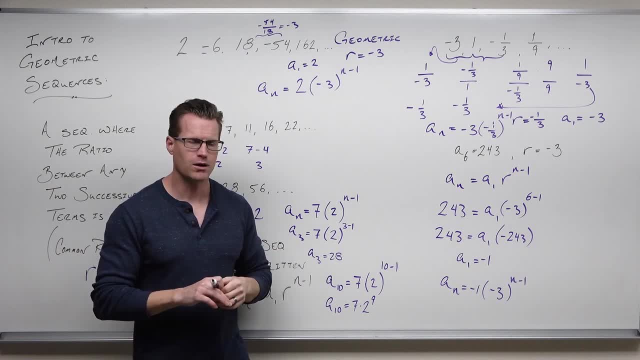 wherever that says to do So, find the seventh term. whatever. We're just plugging in n and using that formula to find the specific term of the sequence. So I'm going to come back with one more and then we'll move on to our series. 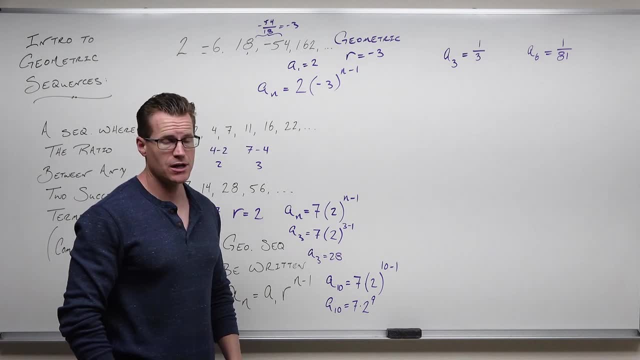 Let's try one more. So what happens when they say you have a geometric sequence but they don't give you the common ratio and you really can't find it easily? We got to set up something from our formula for it and then use not really a system, but some way to set these. 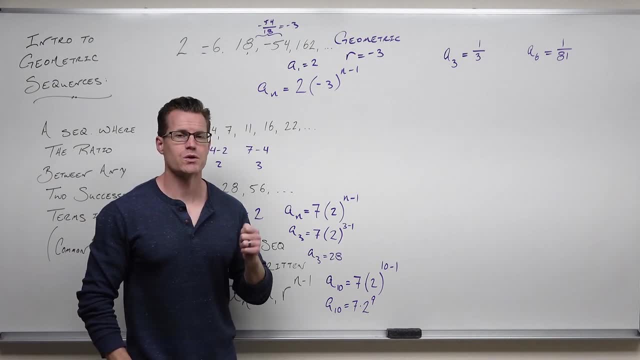 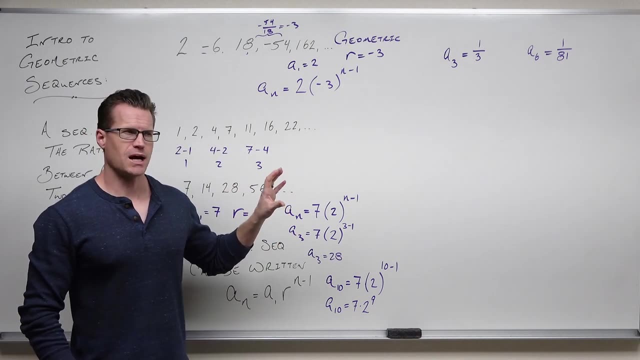 things equal, to find our first term and find your common ratio. So I'm going to show you one way to do this. There are other ways to do it. I'm just showing you one. If you know, this is geometric and it says: I want you to find the formula for it. Let's start. 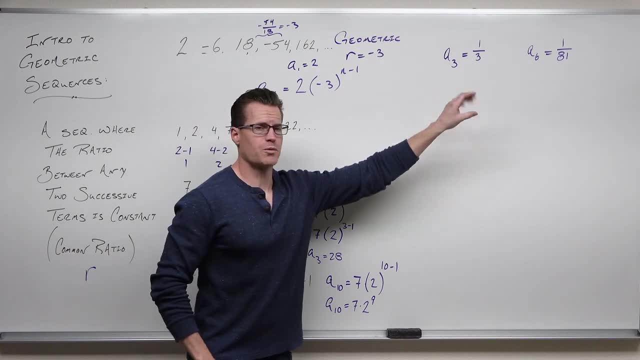 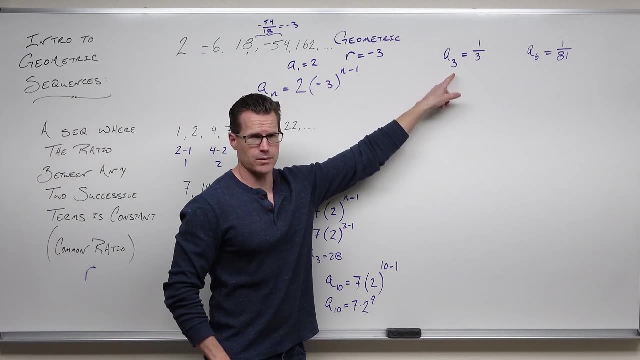 using this and fill it as much as we can for the information we're provided. So, if we know that our nth term is a sub one r to the n minus one and we know a term like a third term and we know the, 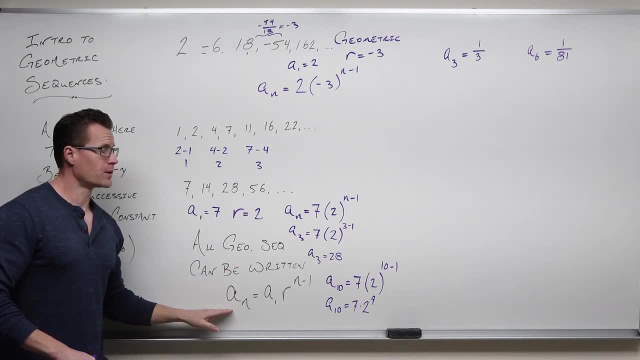 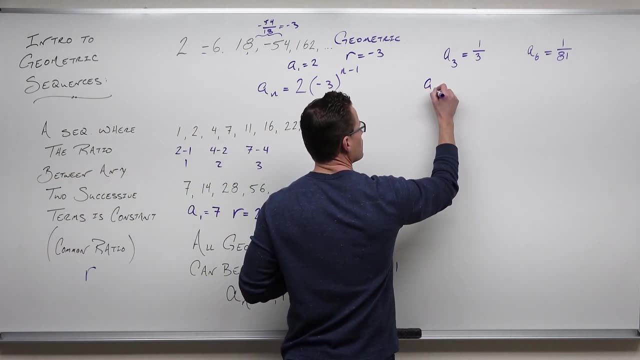 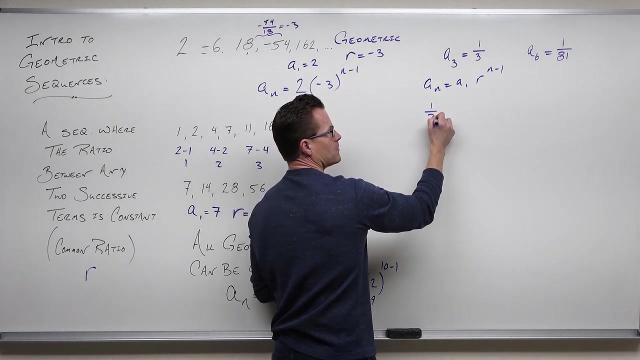 value of it. well, we can set that up. So we know that one third is. I don't know the first term, I don't know the common ratio, but I know that's going to be a three. So one third is our term. I don't know my first term, I don't know my common ratio, but I know this. 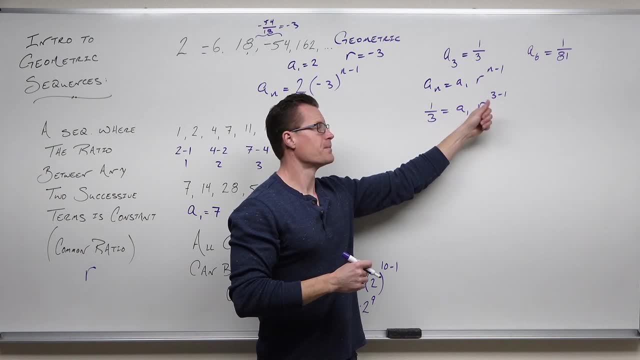 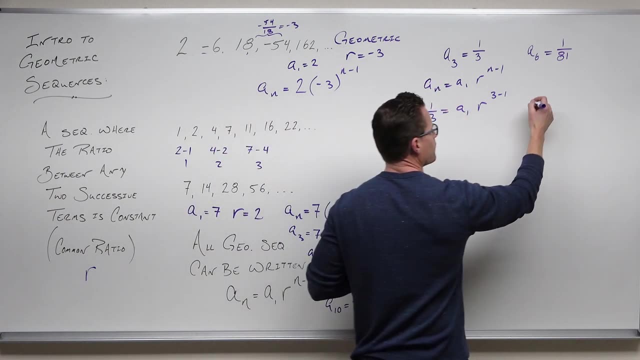 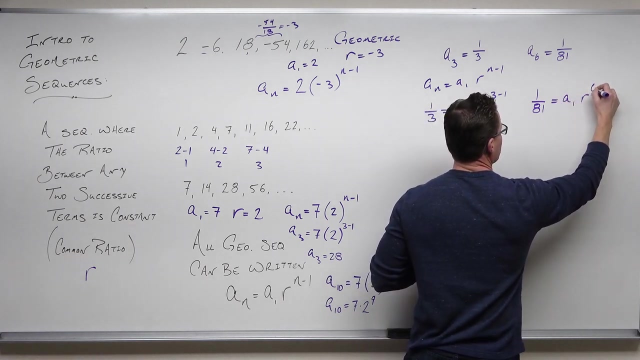 would represent the third term, and we'd have to multiply two iterations of that common ratio to achieve one third. I also have the same or something very similar here, So I know that the six term equals 81. Now I know I still don't know the first term, I still don't know the common ratio. 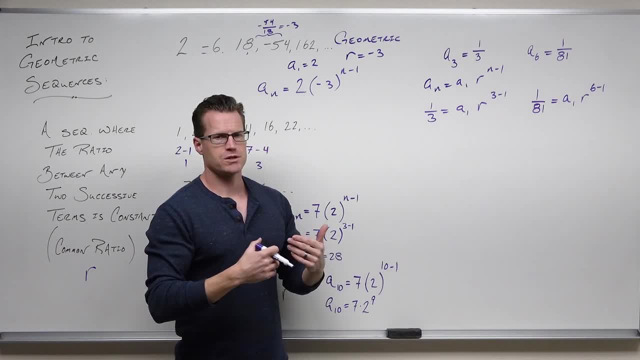 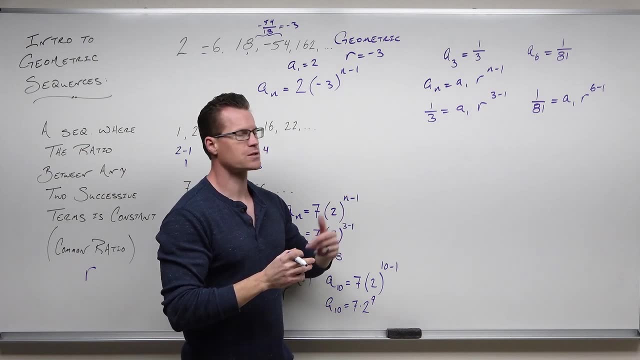 but what we do have here is the ability to set parts of this equal, And so here's what I'm going to do. What I'm going to do is I'm going to solve this, solve both of these for a sub one and set 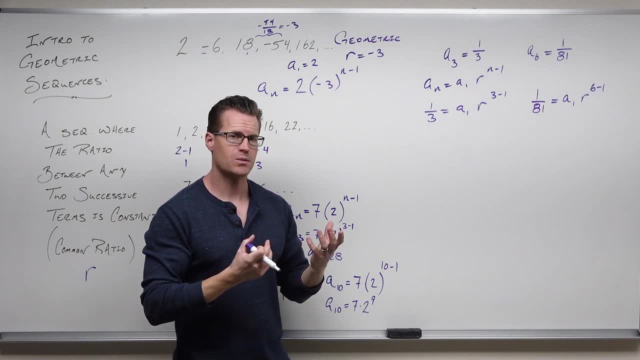 them equal to one another. We can also solve for one and set them equal and divide by a sub one, but it looks a little funny and it feels like you're divided by a variable. You're not, because it's a constant, but I like this a little bit better. It doesn't really matter, but, like I said, there's multiple ways to do. 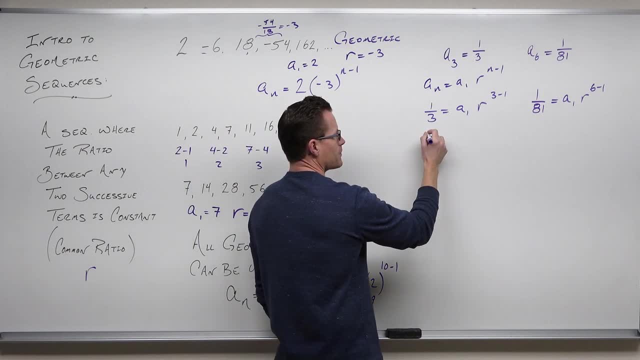 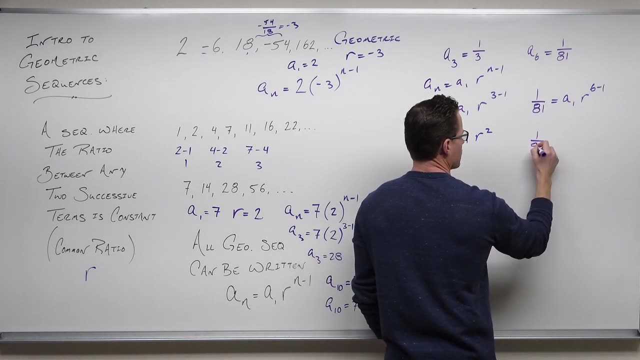 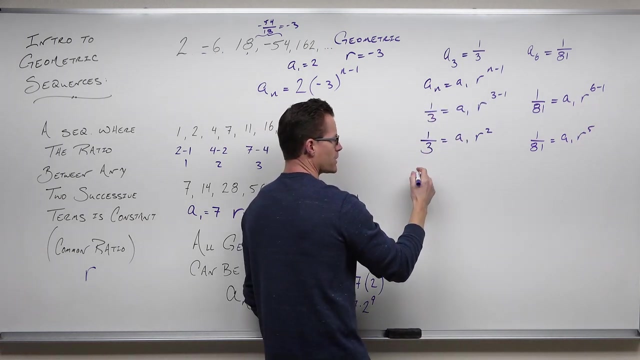 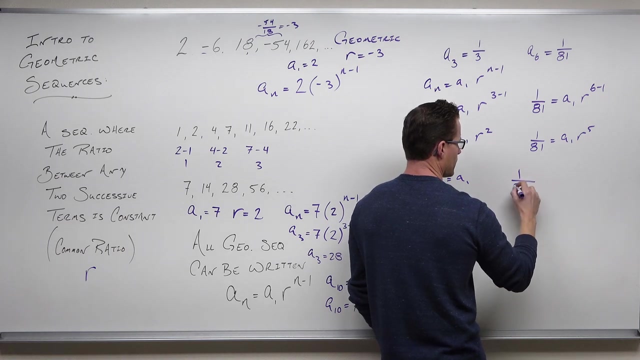 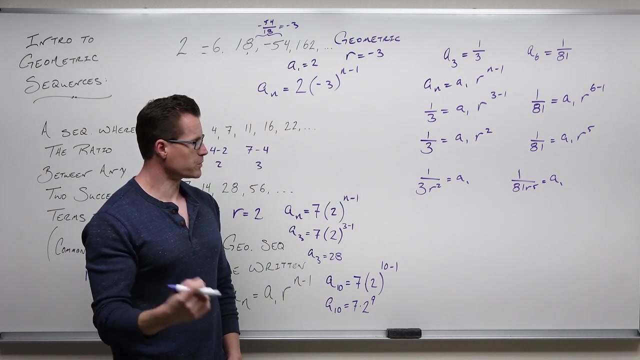 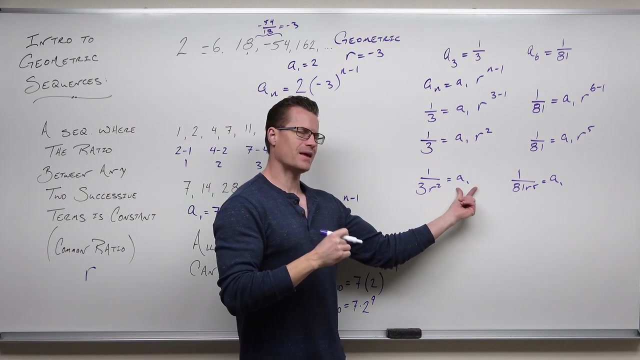 this, but I'm going to solve this for a sub one. So if we do, if we divide by r squared and we divide by r to the fifth, multiple ways, you can solve for this by dividing by different things. But if you have this, and that's the first term, and this, and that's the first term. 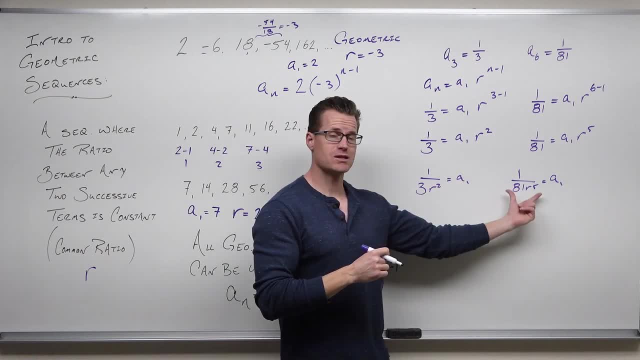 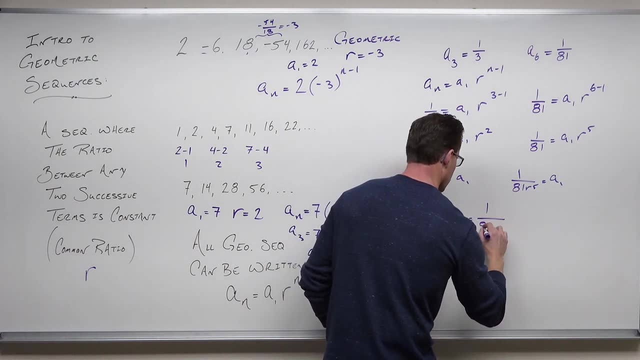 then if you've solved for something you know has to be equal, you can set these two things equal to one another. So now it might look a little funny, but I'm going to solve this for a sub one and I'm going to set 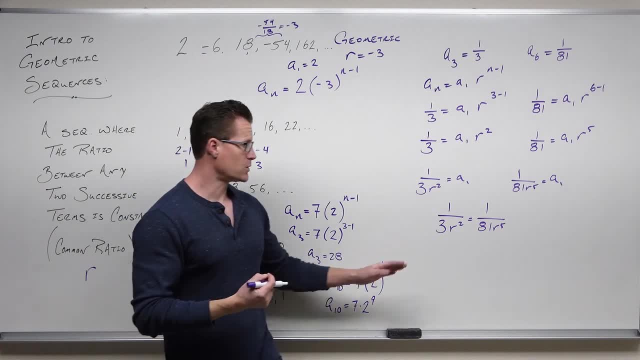 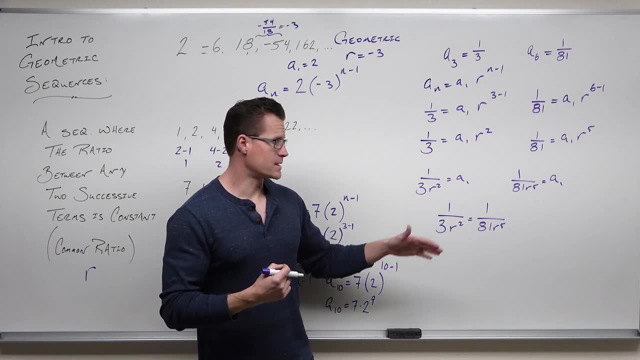 this as a sub one. So think about this: This is a proportion and you can cross, multiply and set equal. So three r squared times one, or one times 81r to the fifth, or realize that one over some variable. 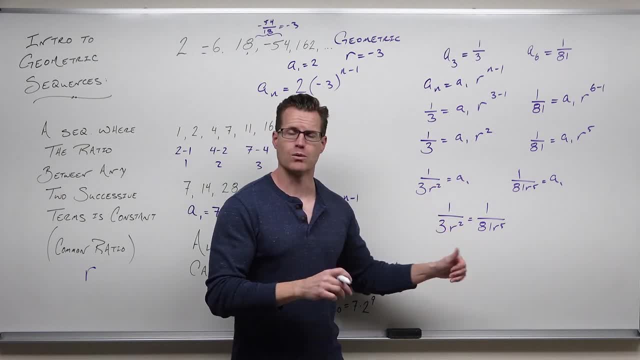 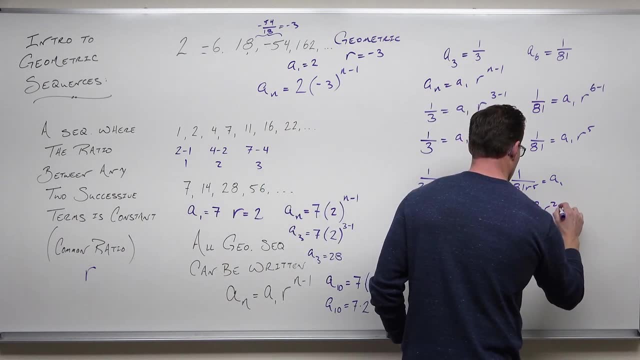 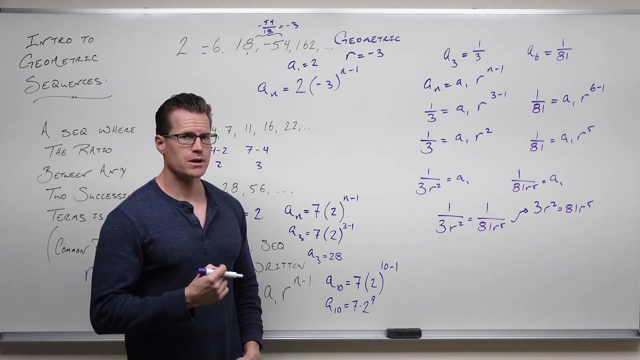 equals one over some other variable. These two variables have to be equal. Any way you go, you're going to get three r squared equals 81r to the fifth. Now what we generally don't want to do with variables. we generally don't like to divide both sides by a variable. 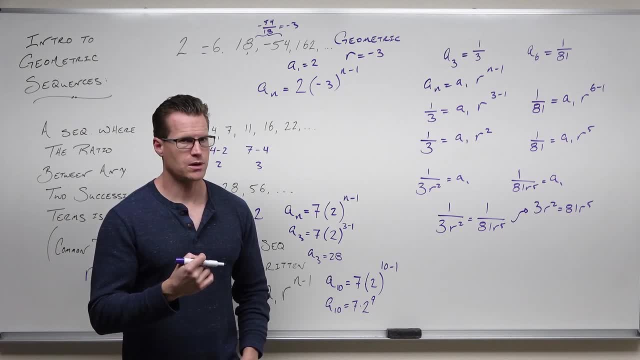 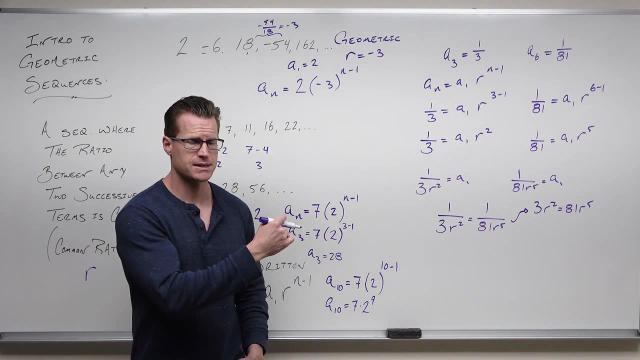 because it could equal zero. Now, our common ratio can't equal zero. It's impossible. It's a constant, It's not zero, because otherwise you would use zero every single time. That's not going to happen. So we are perfectly okay. dividing both sides by three r squared. 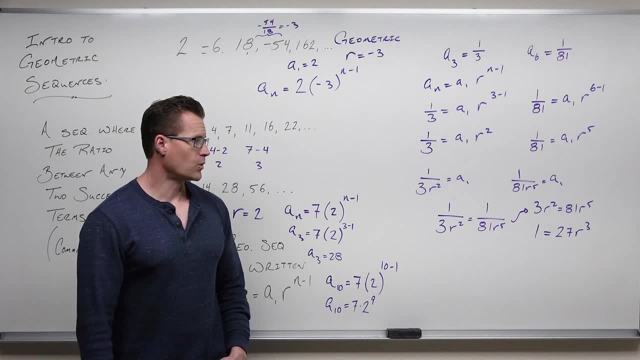 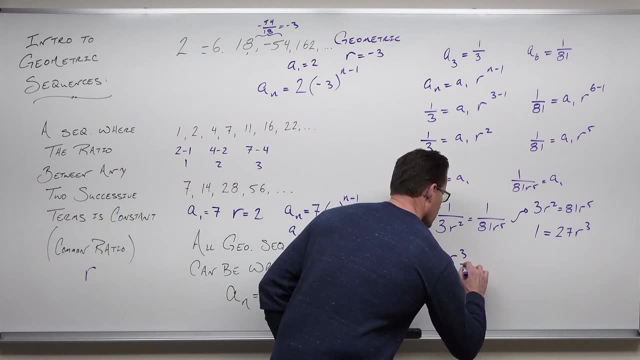 All right, So one equals 27r to the third power. Well, wait a minute, Can you isolate that power three? Yeah sure, Let's divide by 27.. And when we take a cube root, we're going to get one third. 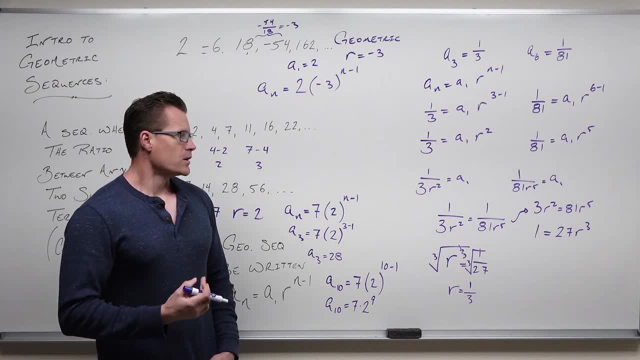 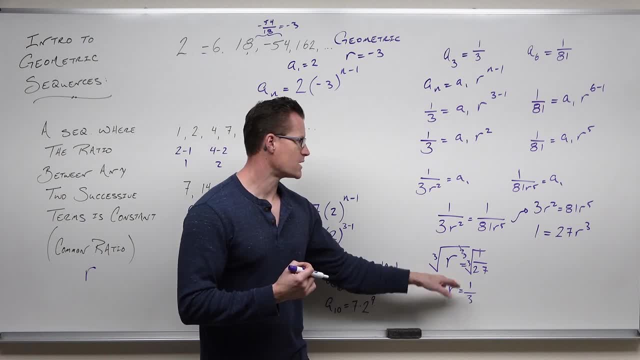 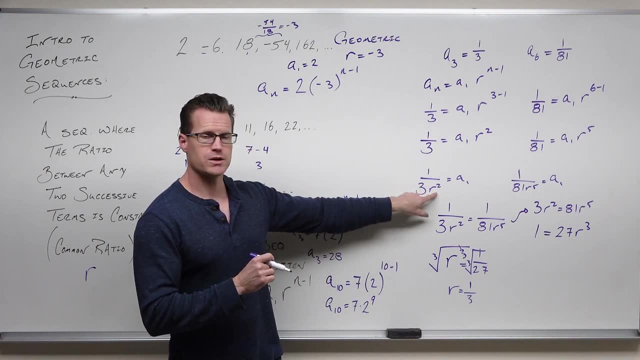 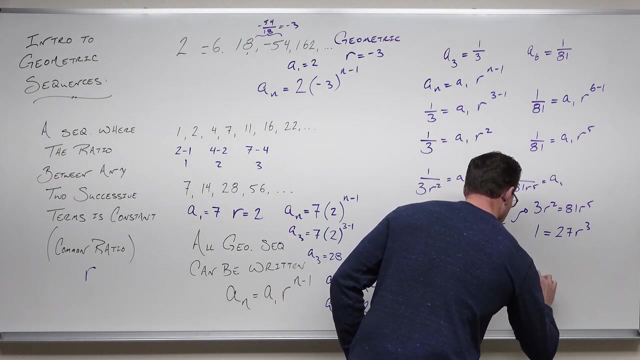 like to write it like this, because it's already solved for you: We just have to plug in one third here. So if we do be careful on your fractions, But if you plug in one third, one third squared is one ninth. So I'm using just like the kind of substitution or system of equations works many. 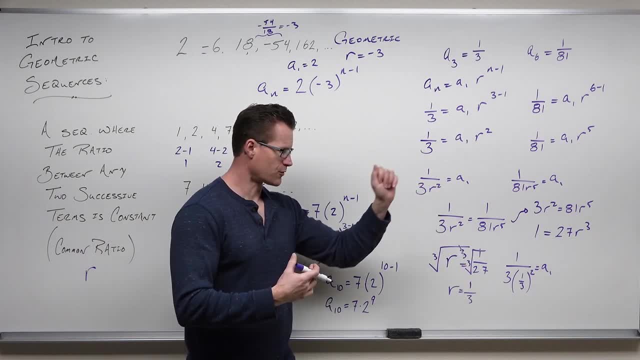 times. I'm using this to solve for a sub one. It's solved for my first term. I'm plugging in my r because now I know it, r squared is one third. So I'm using this to solve for a sub one. It's. 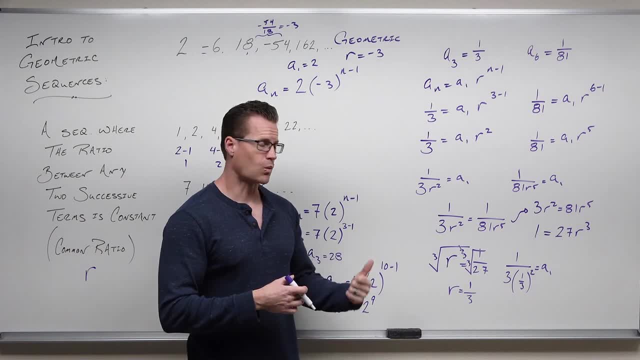 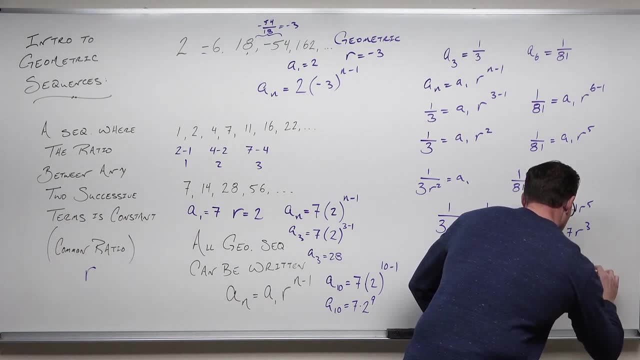 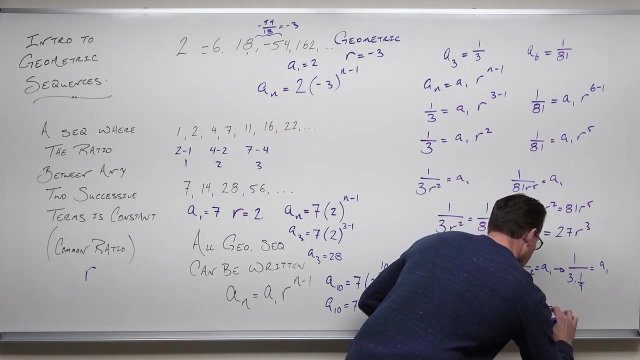 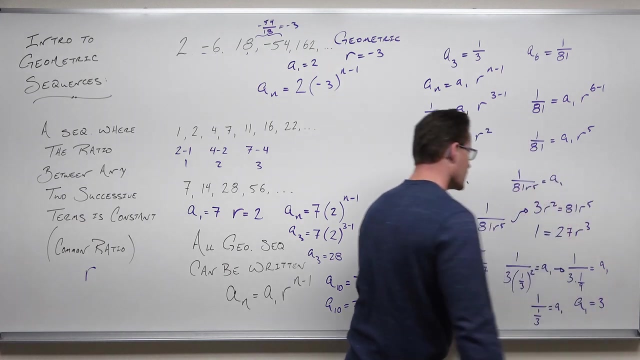 r squared is one ninth Three times one ninth is one third. So one ninth Three times one ninth is one third, And one divided by one third is three. So we now know our common ratio, We now know our first term, And this is pretty easy to. 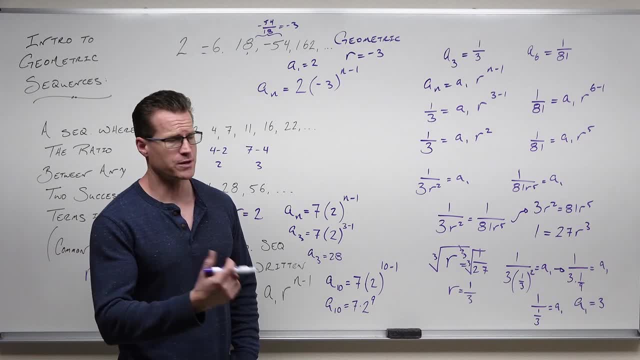 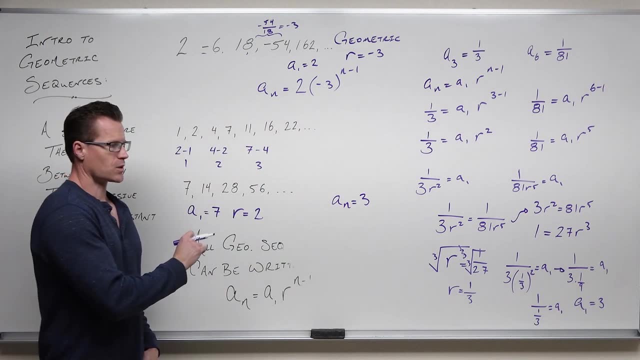 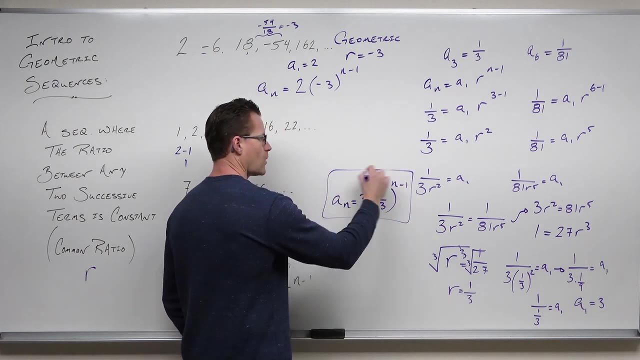 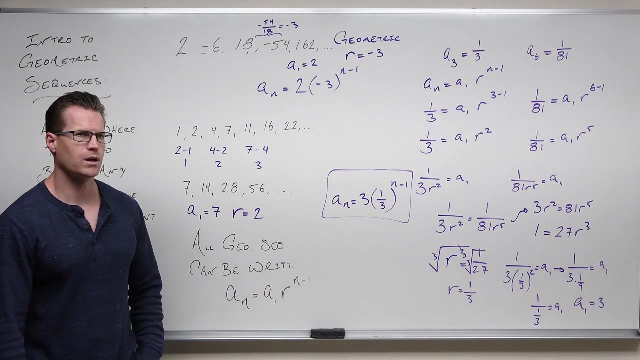 be able to write this as our geometric sequence. So we'd say our geometric sequence is our first term. That's three times our common ratio, That's one third to the n minus one. Now there are some things we can do to manipulate this. I'm not going to do it. You know what? 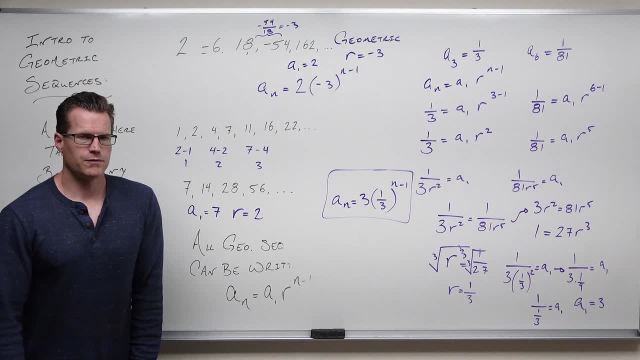 Yeah, I'm going to do it. It's just it gets a little bit confusing for a lot of students. So I'm going to do it. It's just it gets a little bit confusing for a lot of students. However. 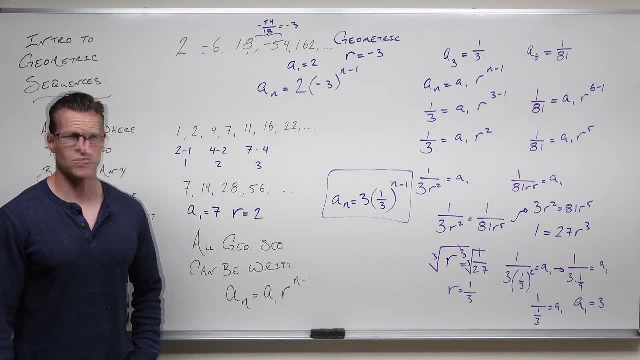 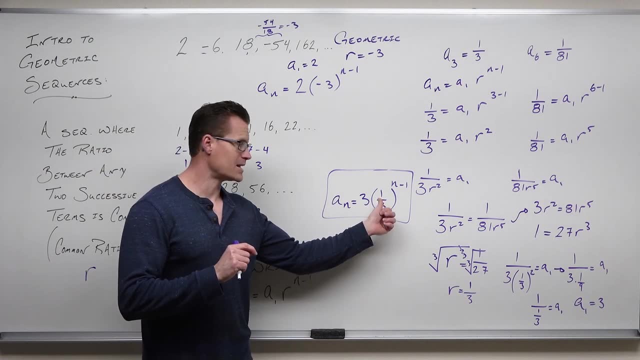 sometimes you're going to see this in the back of your textbook and go: how in the world did we get n minus two? Where'd that come from? Here's where it comes from. If you see a number here and a kind of like a base here that you could somehow make the same, you can combine these via. 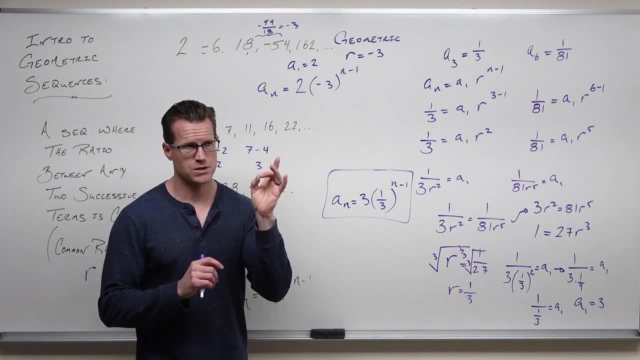 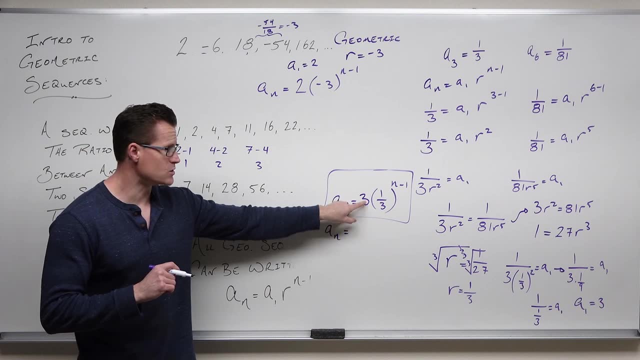 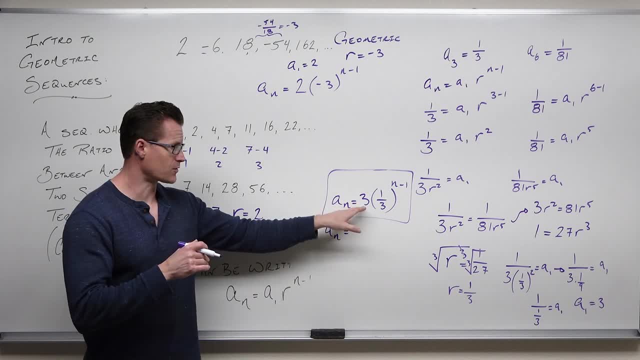 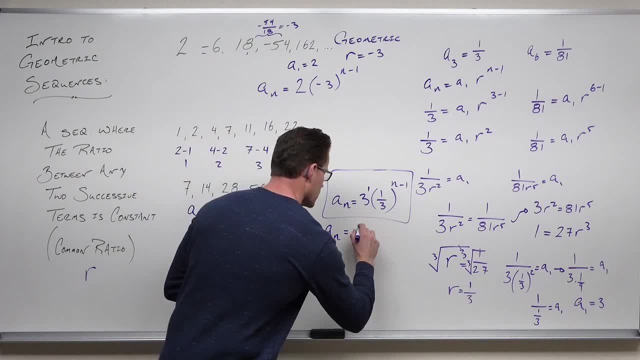 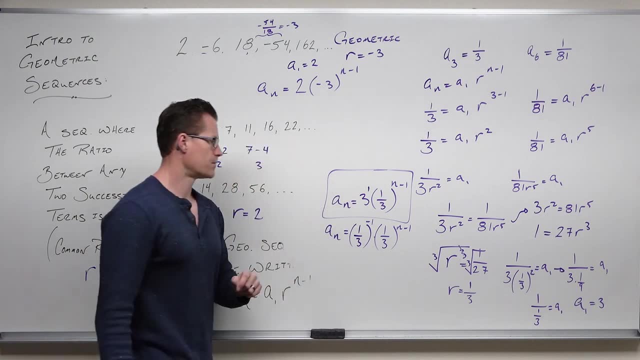 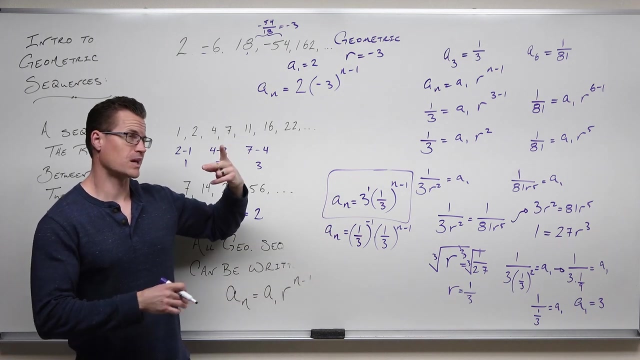 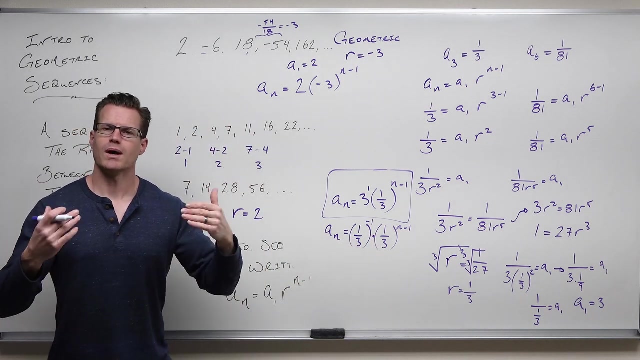 as one third to the negative one. power In your head right now that has to be the same thing as three: One third to the negative one. reciprocate change: the sign is three. but you have it. What do you do when you multiply common bases? You add the exponents. 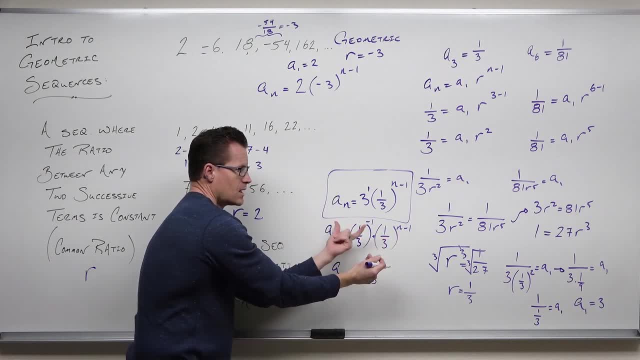 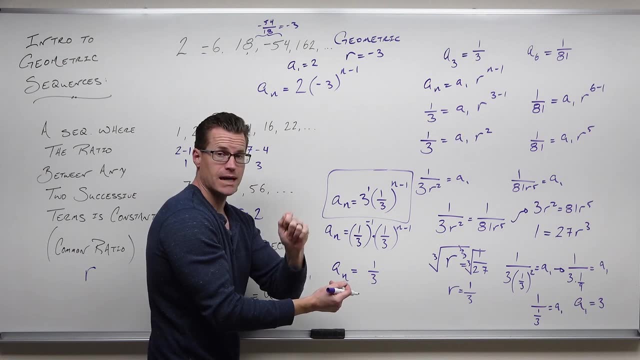 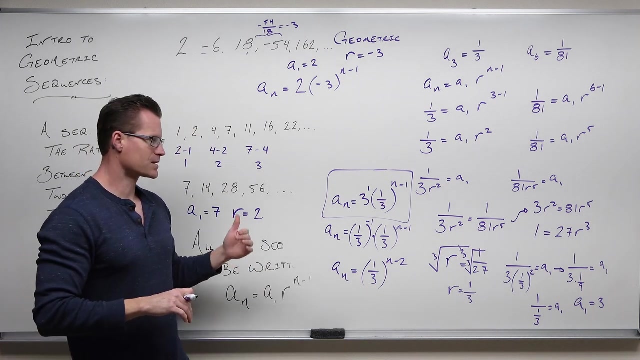 So you could combine these, get the same base- you have the same base- and add your exponents: Negative: 1 plus n minus 1 is not n, it's n minus 2.. And you'll see some of that fancy stuff where sometimes they won't show you this. 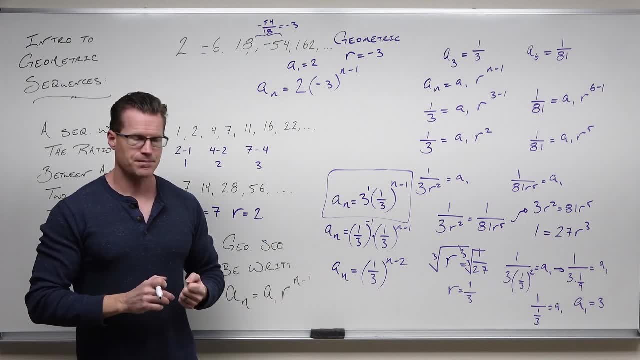 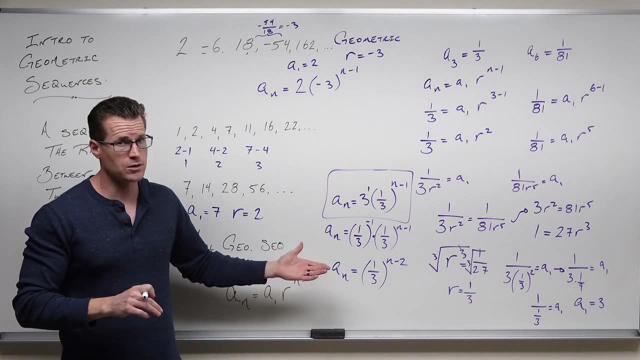 they'll just show you that and you go. I got that. It is the same. This is usually just fine, but sometimes you will see that- and I wanted to mention that to you- It is more concise, right, It is a little bit nicer to work with, but that's where that's coming from. 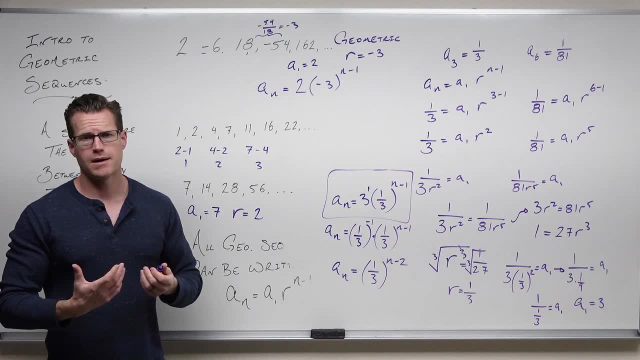 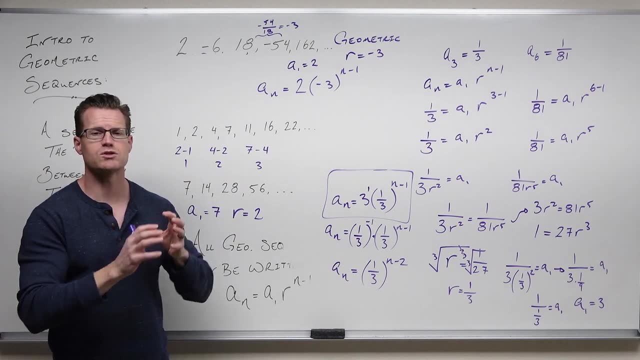 So I hope that you learned in this lesson what a geometric sequence is, that it's similar to arithmetic, but instead of adding, you're multiplying. You can always find a common ratio by dividing all of your successive terms. Just make sure they're the same. You don't want. 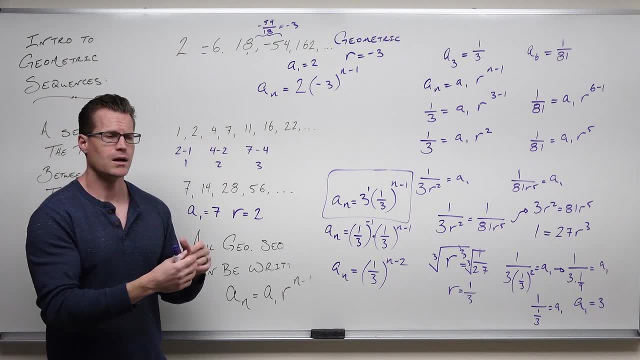 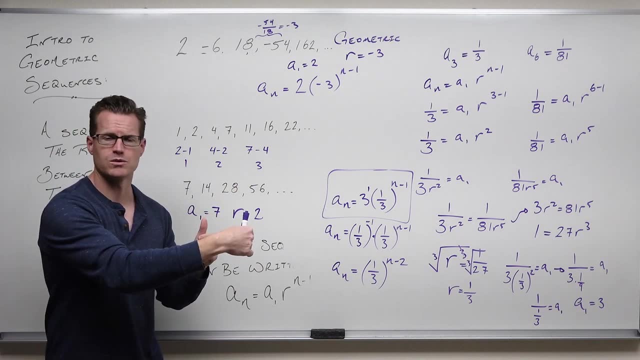 to stop after 2 and assume you're right. You really want to check The formula is really easy. Just have your first term. have your common ratio with n minus 1.. The n minus 1 is there because we need one less iteration of multiplication to get the term that we want. 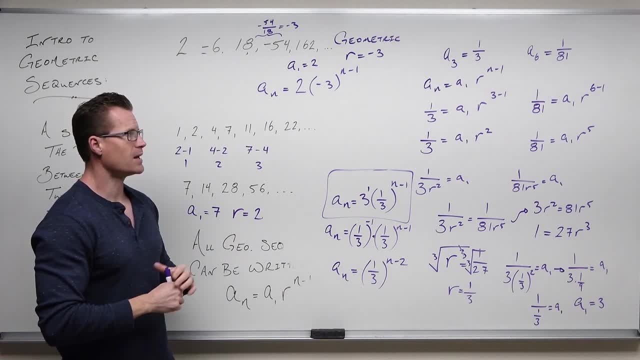 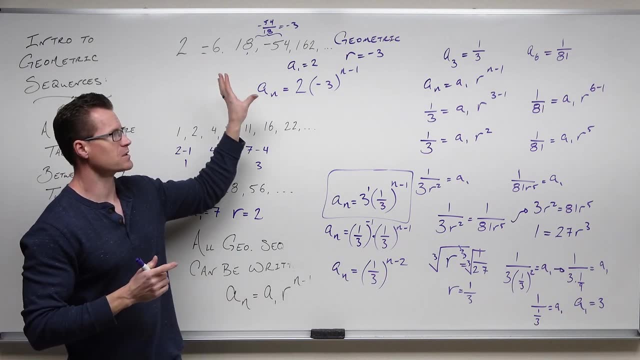 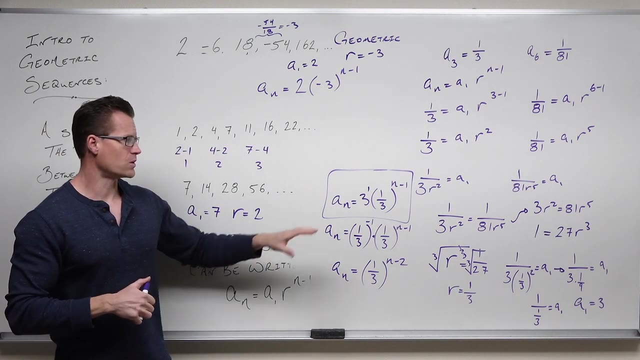 considering that our first term is taken up by a sub 1.. After that, I've given you as many examples as I could find or come up with about how to create a geometric sequence just from either some sequences themselves or knowing one term or several terms. After that, I've shown 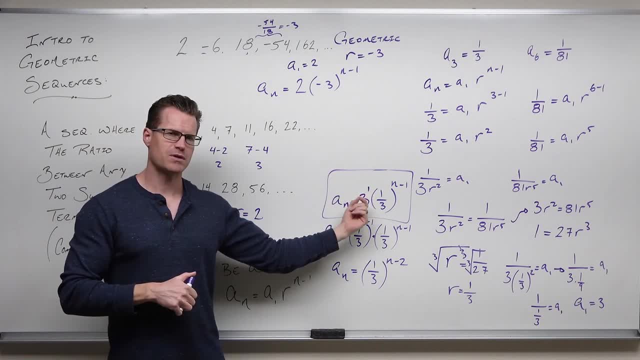 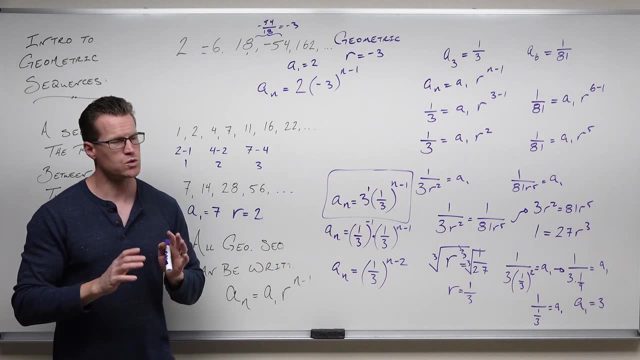 you a way to take and make more concise some of these geometric sequences. when they have a first term, that can be written as your common ratio. Usually it's with a negative exponent, Usually it subtracts here. somehow It can be a positive exponent, It's just usually not. 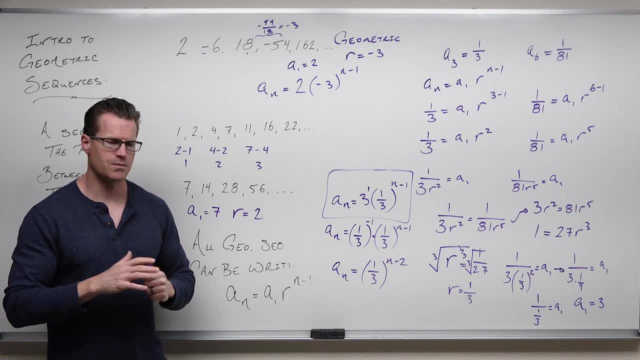 and then you get that n minus 2.. So I hope it makes sense. What we're going to do now is come back with a geometric series and learn how to add these sequences up. 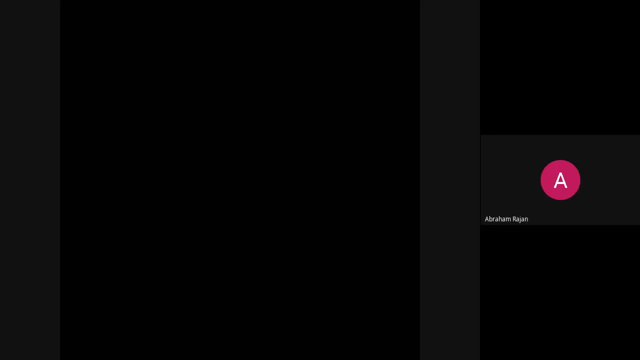 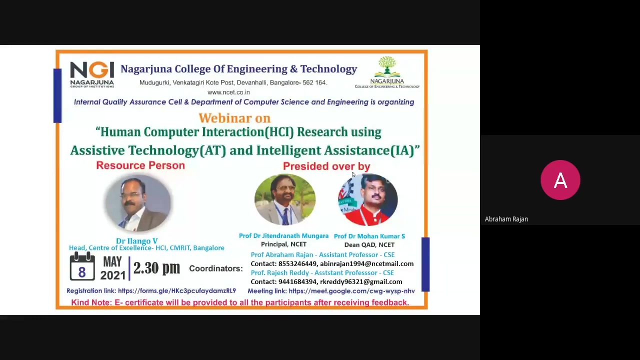 A very good afternoon to one and all present here. It's a wonderful day and I feel privileged to extend my warm welcome to beloved Professor Dr Jitendra Mungar, sir Principal of NCET, and Professor Dr Mohan Kumar, sir Dean of Quality Assurance Department, NCET and our resource. 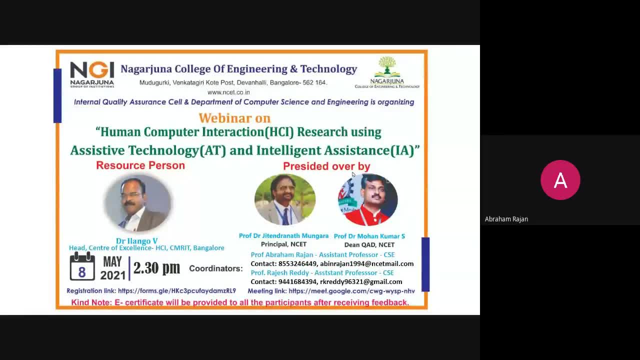 person and speaker of the day, Dr V Longo. sir, Head Center of Excellence, CMRIT Bangalore. I would also like to welcome all HODs, faculty members and all participants. Today we have gathered here for a webinar on Human-Computer Interaction: Research using Assistive Technology.